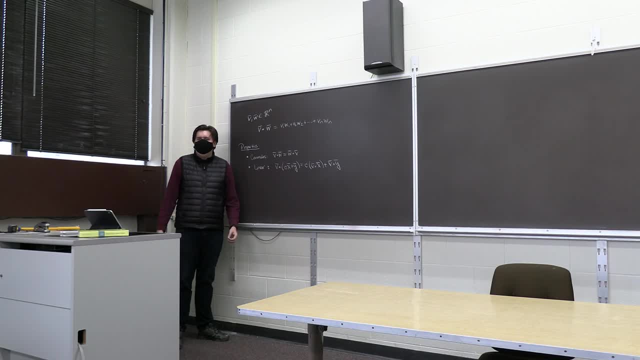 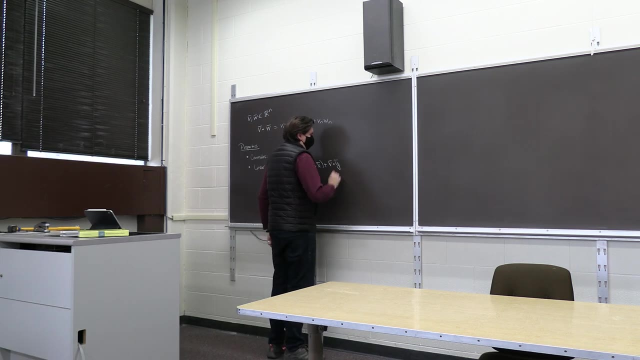 Why? Because it commutes. So if you want to show it's linear in the first argument, you would just use the commutative property, Then use that it's linear in the second and then bring it back right. So these two together actually give you that it's bilinear. 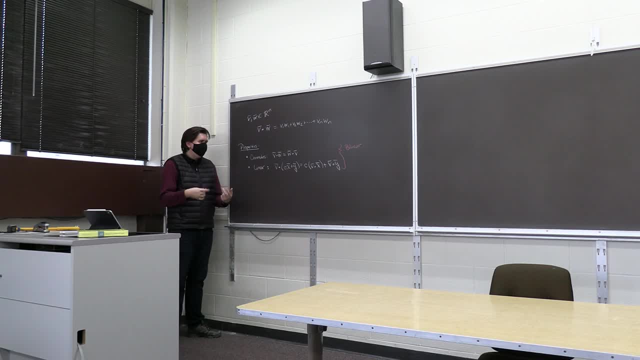 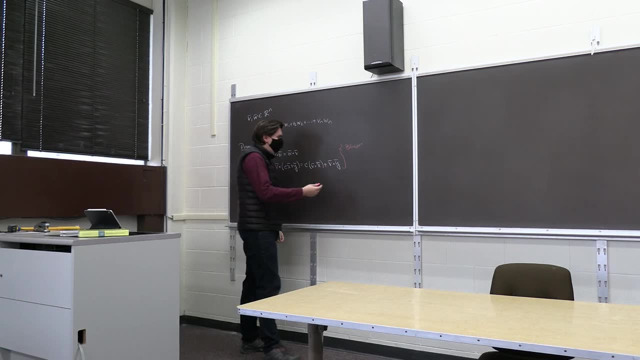 I mean I could just say it's bilinear. but I'm trying to make the point that we can be a little bit more conservative when we say: and this falls out. So if that's not clear, let me just make this explicit. 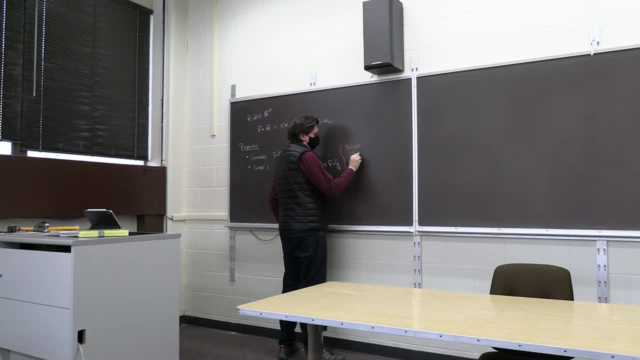 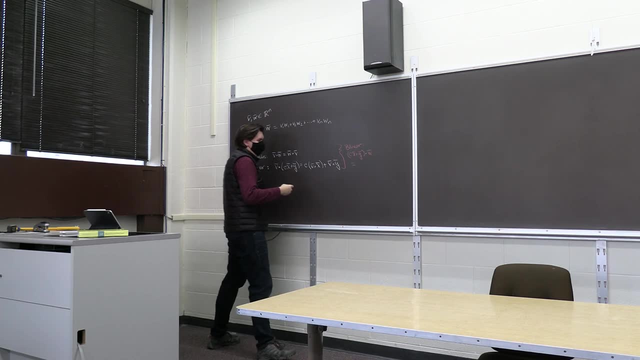 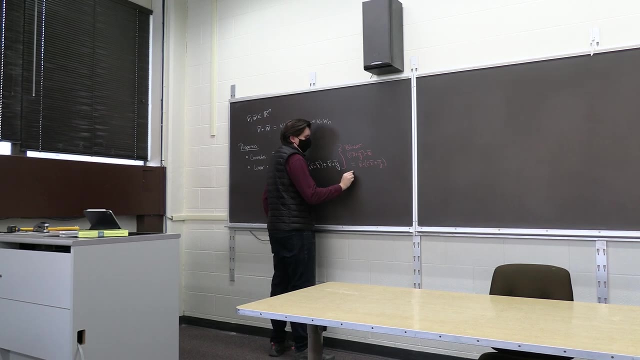 If I wanted to you know, cx plus y dot w, v dot. x plus y dot w. The way we do that is first we use the commutative property to say that's w, dot, cx plus y, And then we use this linear in the second term. 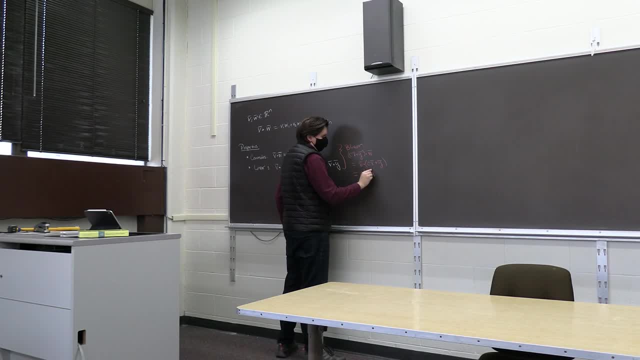 So that's c times w dot x plus w dot y, And then we use the commutative property again, right? So this is c x dot w, So w dot x plus y dot w. w dot x is the same thing as x dot w because it commutes. 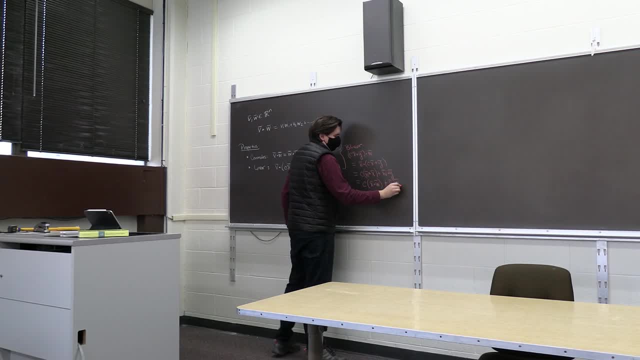 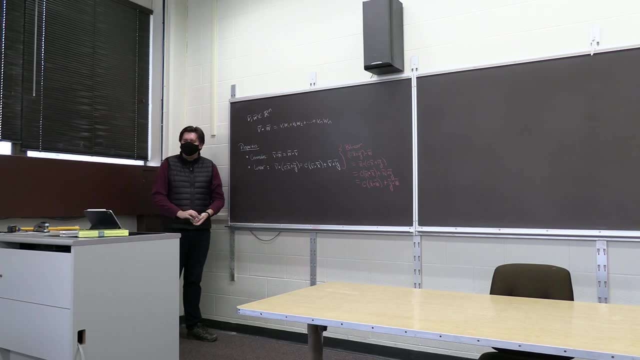 And w dot y is the same thing as y dot w, So that's how those two properties work together to give you that's also linear in the first argument. Okay, nice. So whenever you have something that's linear in one argument and that's commutative, you actually have it's bilinear. 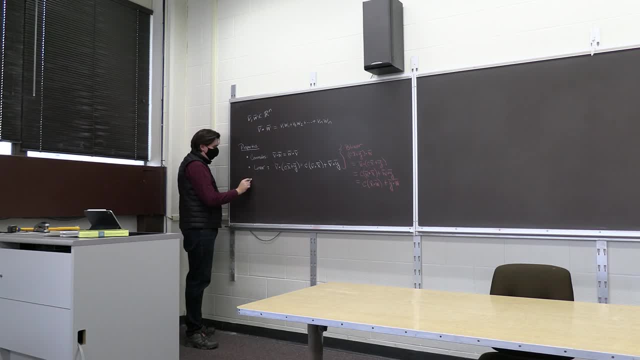 And maybe the last thing I'll say about the dot product, which used quite a bit in introduction to linear algebra, which used quite a bit in introduction to linear algebra, which used quite a bit in introduction to linear algebra, is that it's positive, definite. 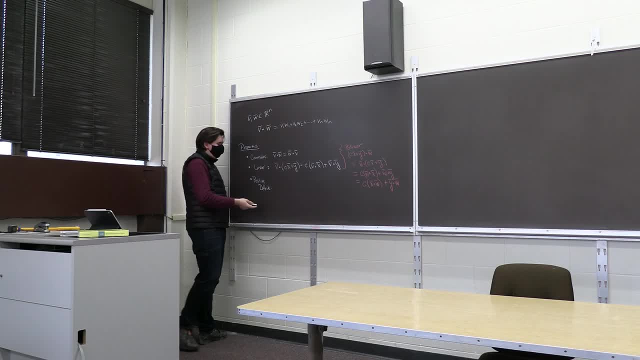 So we call it positive. definite means: if you take some vector v and you dot it with itself, this is always going to be a non-negative value, Like just think what this guy is. This is just the first value of v. So v is v1 through vn. 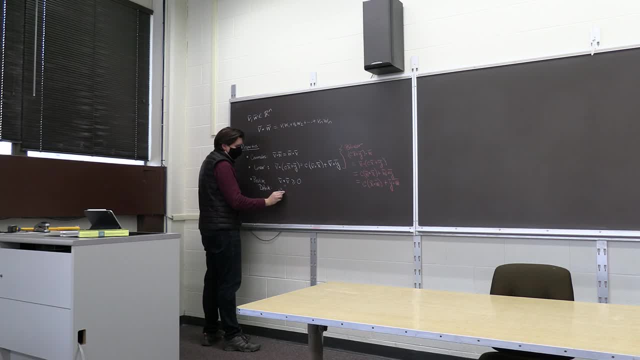 That's just v1 times v1.. So v1 squared up through, vn squared Right. So it's like: yep, that's always non-negative, In fact, something a little bit stronger- is true, It's always non-negative and it's equal to 0. only when, if and only if. what? 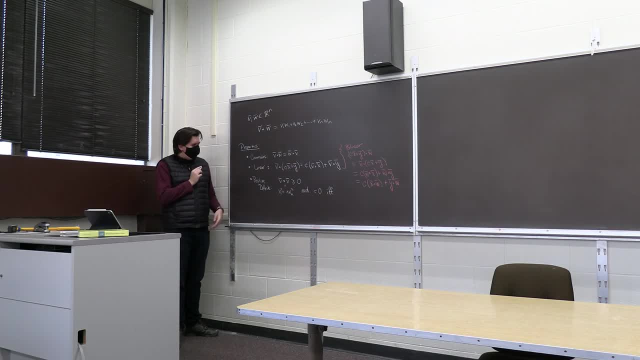 Yeah, it's like. the only time for a sum of squares to equal 0 is if each value is itself 0. Right, Which means v itself must be 0. If, and only if, v is 0.. So this is what I mean by positive definite. 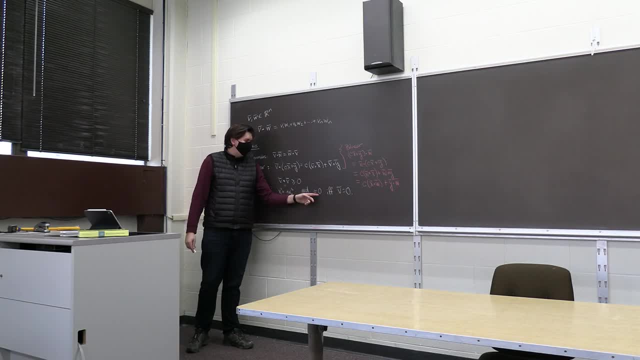 It's always positive, except for the case where you have the 0 vector. then it comes out to be 0.. Okay, this term is used lots of times. You can talk about positive definite matrices. You can talk about all kinds of things being positive definite. 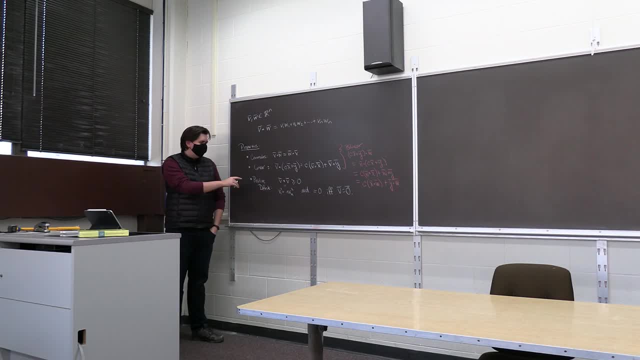 But in general, in particular, the dot product is positive, definite. So it's like: why is this nice? Well, this kind of then leads into. so it's these properties of the dot product that tell you the dot products are a really useful thing. 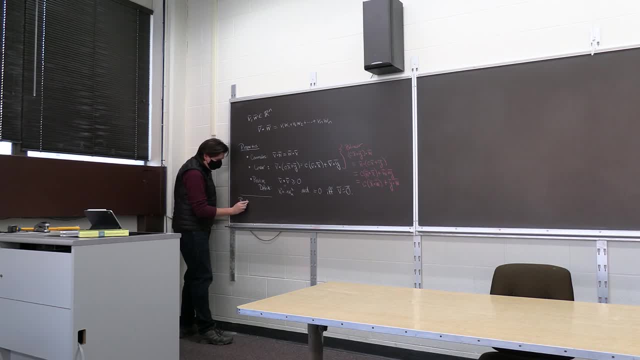 Right. So in your first course on linear algebra, and I suppose also like in multivalve calculus, you become convinced that the dot product is really nice. So what kinds of things does the dot product tell you? Okay, great orthogonality. 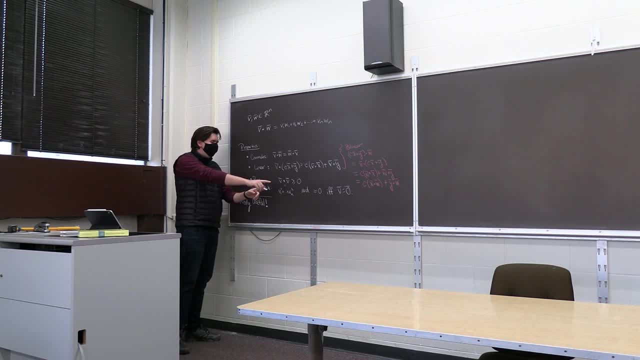 So let's get there in a second. In order to have a notion of orthogonality, we're first going to introduce the notion of a length or a magnitude, Right, And so one thing you first learn is the magnitude of a vector. 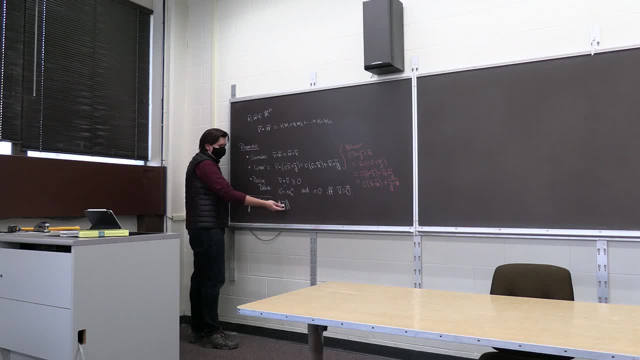 can be defined in terms of if it's dot product. If the magnitude is just v1 squared through vn squared square rooted, we can define this as just the square root of v dot itself. Right, So it's like you can use the dot product. 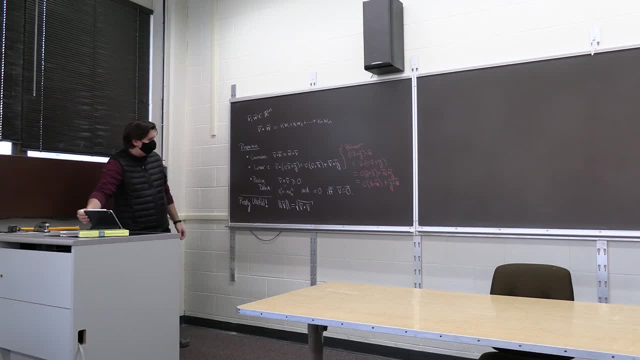 to figure out what is the length or magnitude of a vector. And then you have this really beautiful result where you're like, if you have two vectors in Rn, v and w, not only can we use the dot product to determine the magnitude of both v and w, 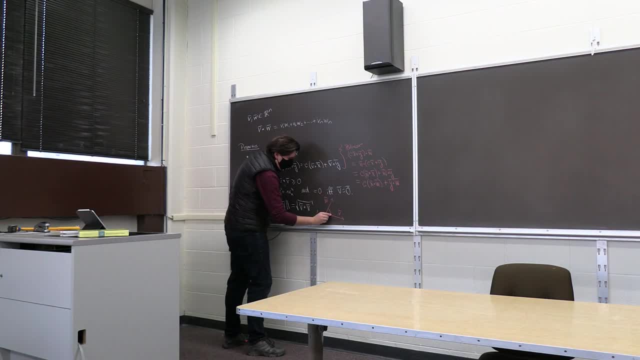 we could also use the dot product to figure out the angle between them. So do you remember what this relation was? This is in Rn right? This is just recalling from your first course in algebra. maybe some multivalve calculus that shows up. 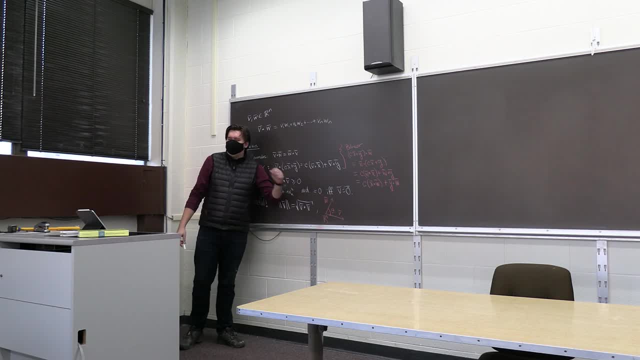 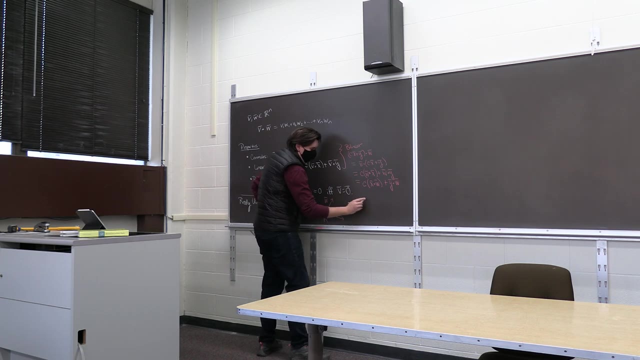 What's the relationship between v, w and this angle, in terms of the dot product, v, dot, w is: you'll have the magnitude of v, you'll have the magnitude of w and you'll have cosine theta, Cosine theta. 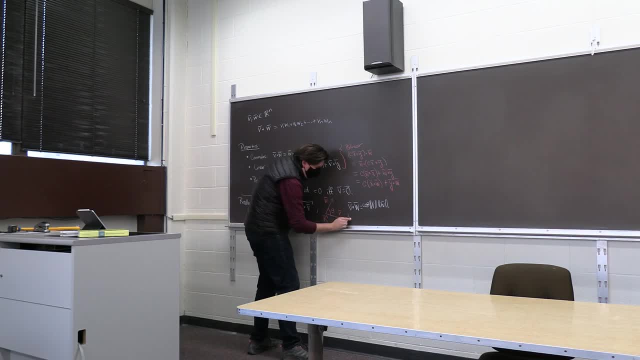 Which, in particular, tells you that if v and w are orthogonal, if your v and w are orthogonal, that is like perpendicular to each other, right? Then what is cosine of theta going to be? Well, cosine of pi over 2 or 90 degrees is 0. 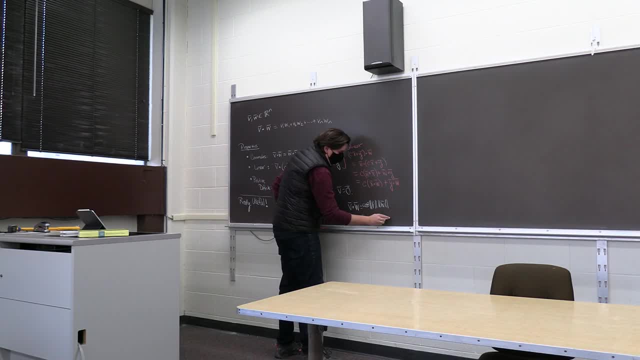 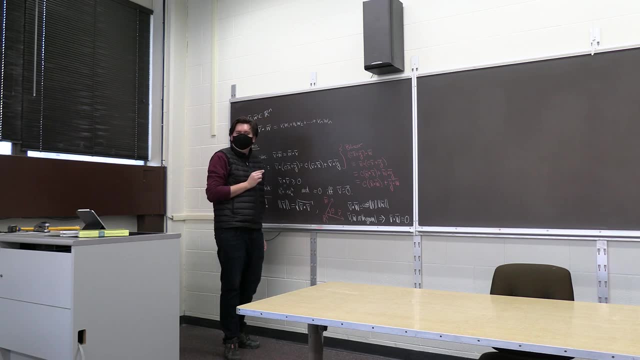 So when you have orthogonal vectors, your dot product gives you 0. And I suppose it goes the other way too. You could have v or w be the 0 vector, and then I suppose you could define the 0 vector to be orthogonal to anything. 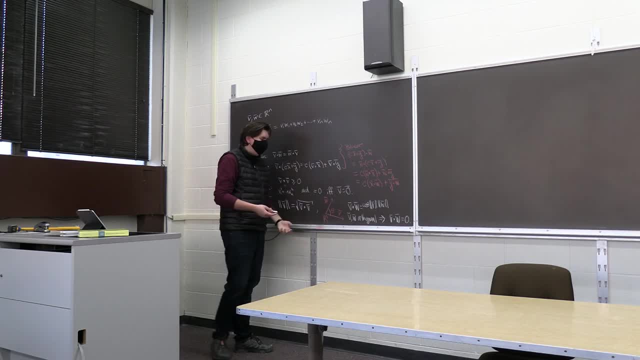 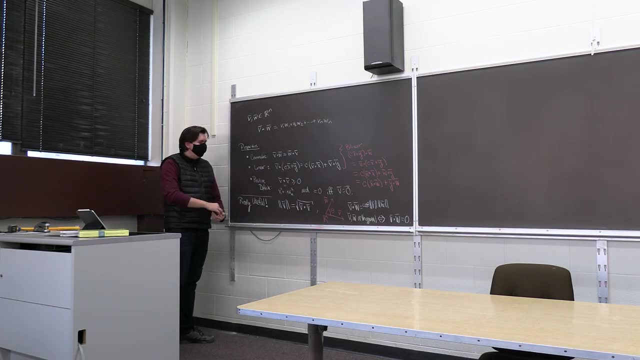 So what this is saying is: the dot product is a way of detecting if something is orthogonal, Or just the trivial 0 vector, right, Okay, So it's really useful in Rn. So what we want to do is we want to ask. 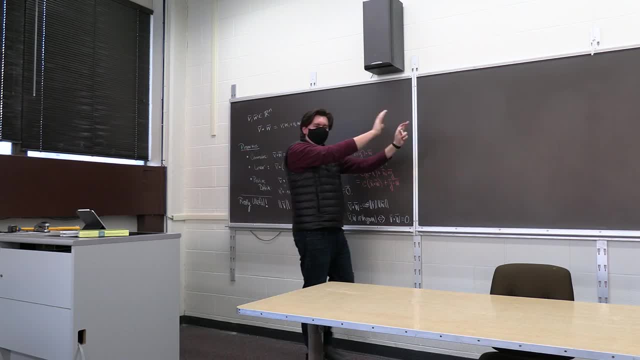 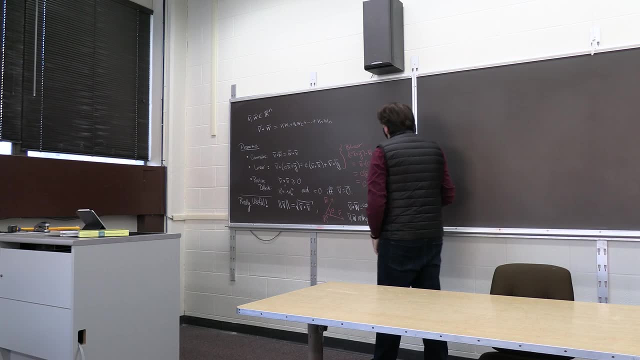 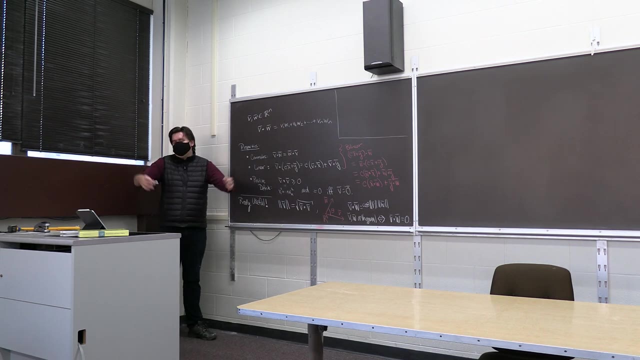 can we take this idea of dot product and generalize it to arbitrary vector spaces? And one way we've already started doing this a little bit is it's like: well, you know like what if my vector space is like some space of polynomials? 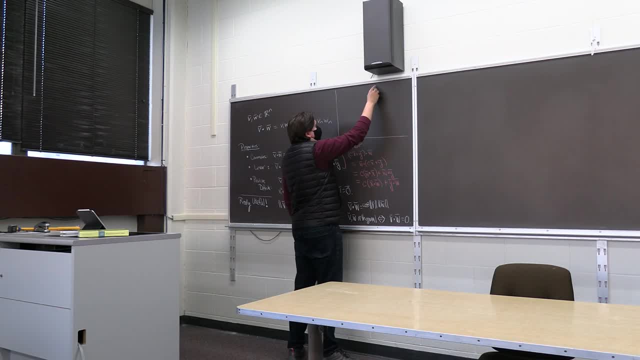 What if I have, like I don't know, like vectors inside of p3?? And so you know what is? two vectors in p3?? Well, maybe like x cubed minus 1, and something like x squared plus 2x plus 1.. 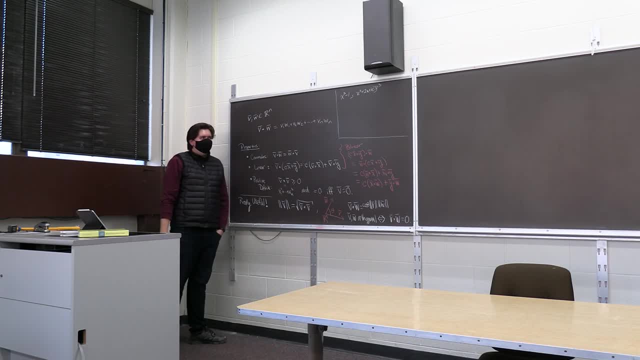 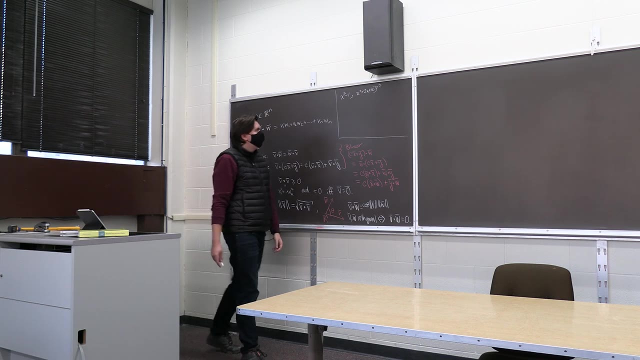 So those are both vectors in p3. And it's like, well, what does it mean to dot to you know, polynomials Like that's kind of weird. Well, the way we think about it before is we say there's a natural map. 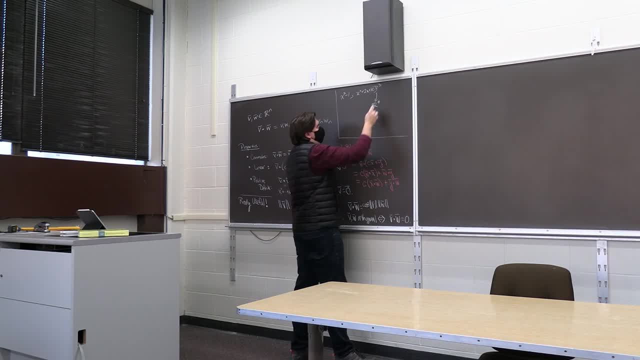 from p3 to R4, where you just remember the basis of p3, the standard basis is 1x, x squared, x cubed, And so then you can just look at your coefficient vector in terms of the basis b. So this guy, for instance, 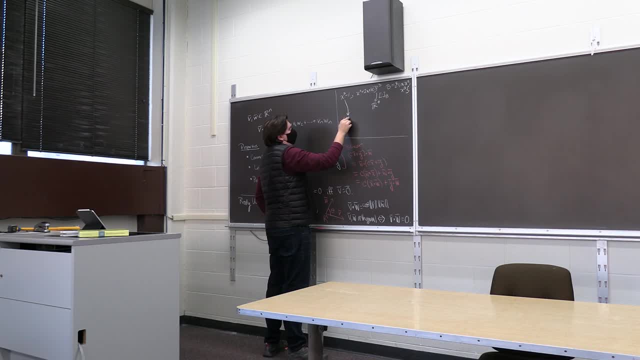 has a coefficient vector of negative 1, zero x's, zero x squared's and one x cubed. This guy has a coefficient vector of one, one, two x's, one x squared and no x cubed's. And then now 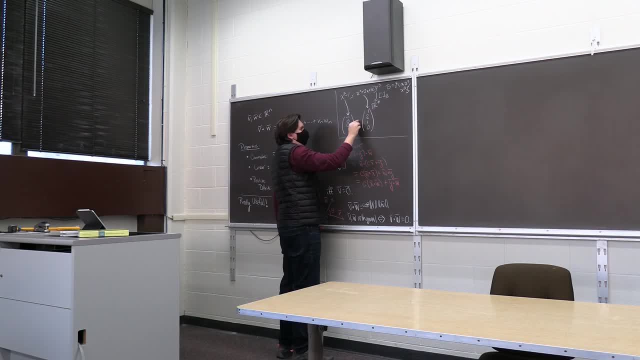 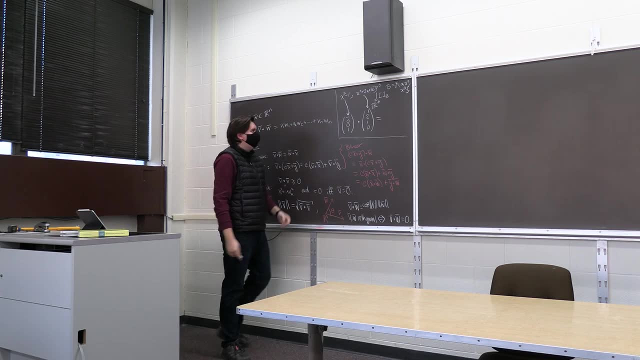 now you're in R4, and so since we're now in R4, we can dot these together and you can get you know, just do the regular dot product in Rn And it comes out to be negative 1.. 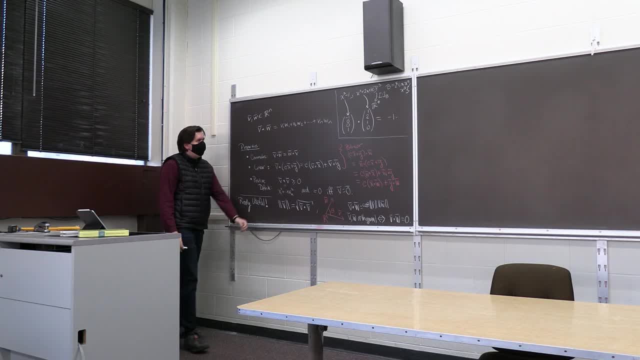 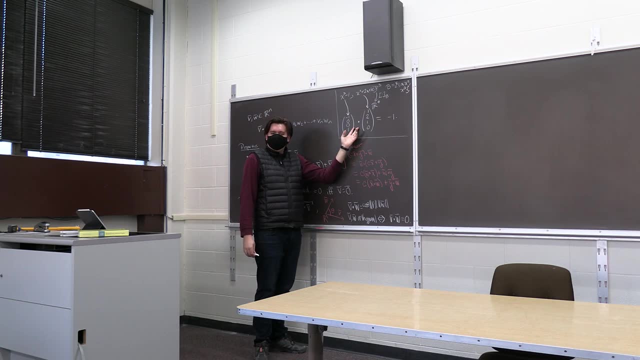 So we already have that story. You can take any vectors in a finite dimensional vector space, find the coefficient vectors in terms of some standard basis- whatever your basis is- and then find the dot product. But it's like two reasons why this might be unsatisfactory. 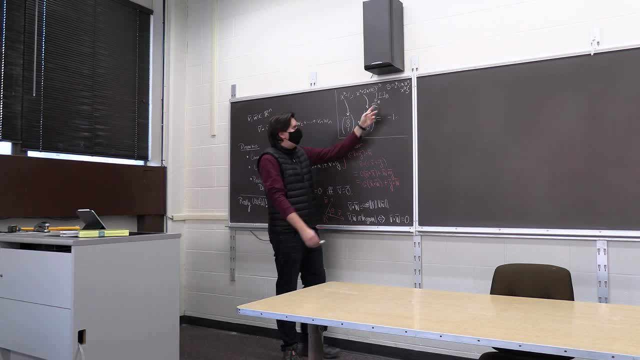 Reason one is this is dependent upon your choice of basis. If I picked a different basis, these coefficient vectors would be different, right? And so you might worry like maybe, maybe it's a little bit less interesting, right? Like it's not so inherent. 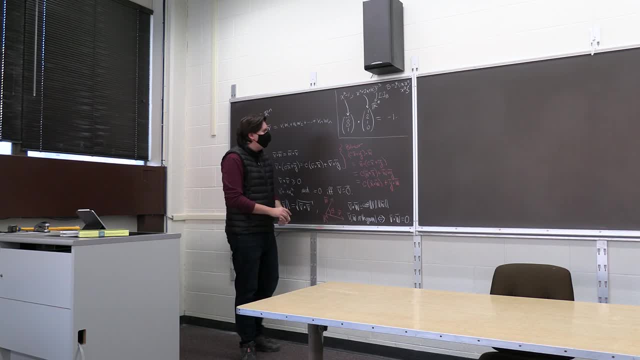 to your vector space. It's kind of just based on whatever your choice of basis is. You could ask, as you change basis, what properties stay the same, What change? Like? those are questions I'm good to ask, But like the second and perhaps even more, 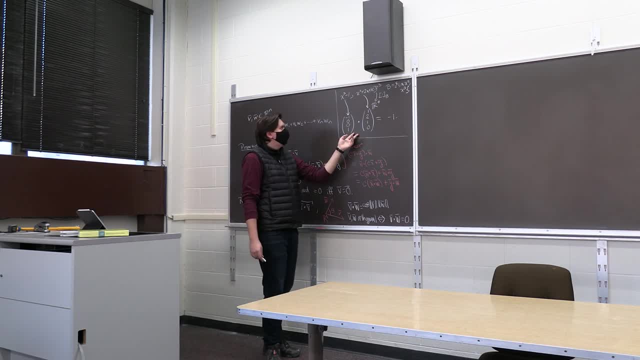 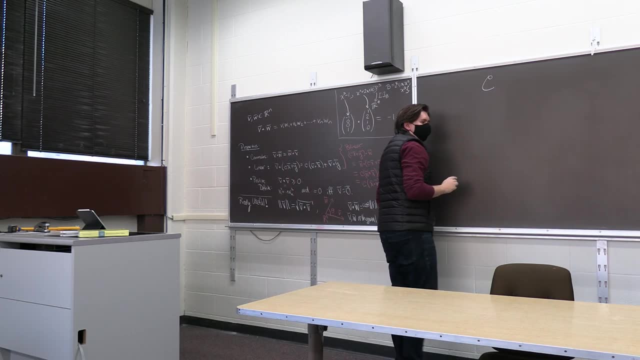 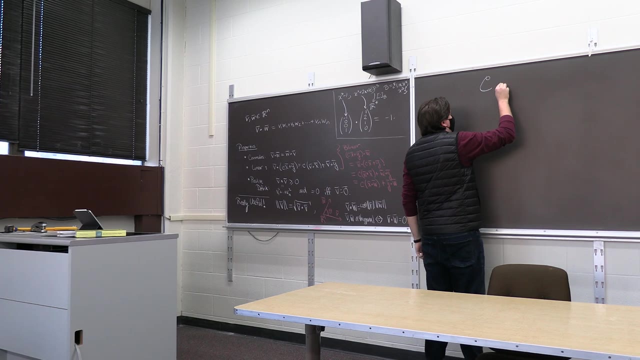 fundamental problem is: this only works if you're in a finite dimensional vector space. What if I, you know, am in some vector space like C, The vector space which is all continuous functions? Right. So this is my vector space, Which is the space. 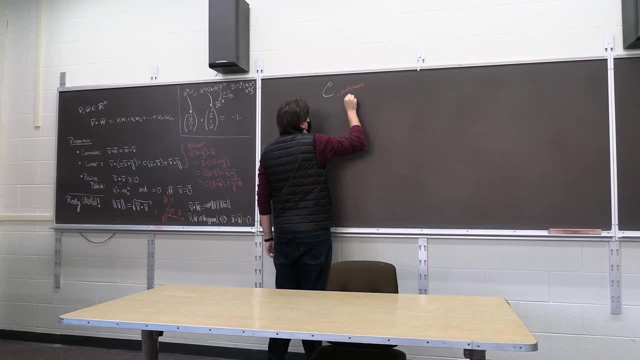 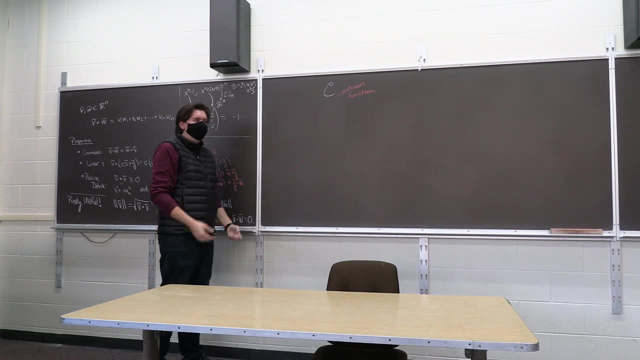 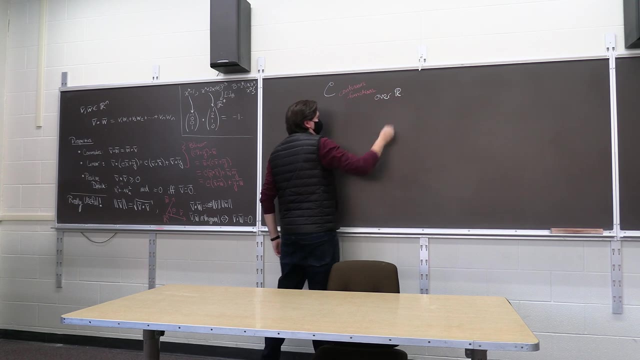 of continuous functions. You can add two continuous functions, get a continuous function. You can scale it by a real number, So let's make these like real values. So this is like over r, Still a continuous function. There's a zero function. 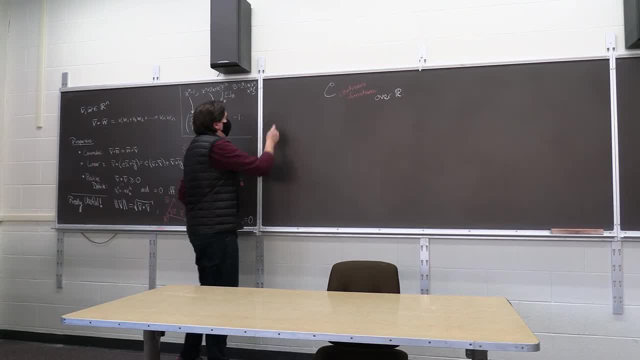 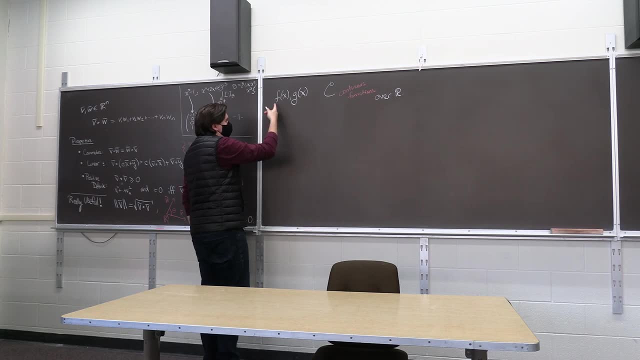 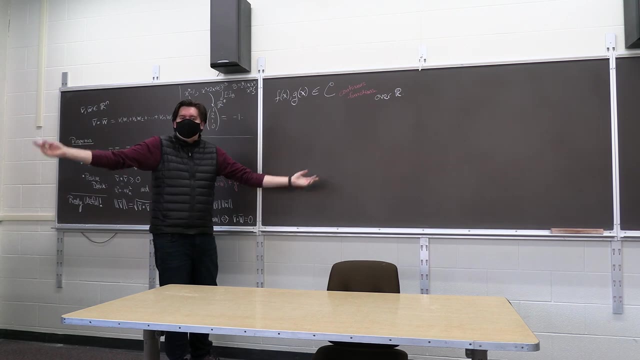 Like it has all the properties of a vector space. And what if I have just two vectors, which for us would be just two continuous functions, f and g? You know, maybe f is something like e to the x, Maybe g is something like cosine of x, Whatever, 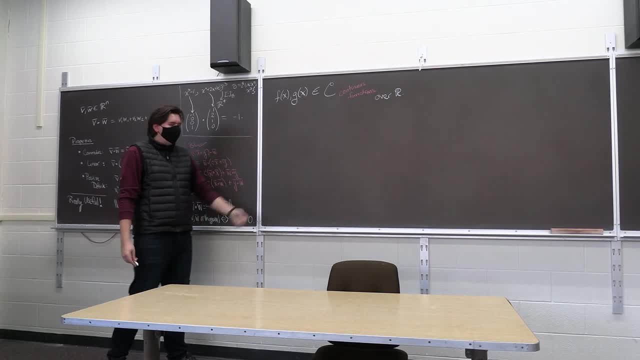 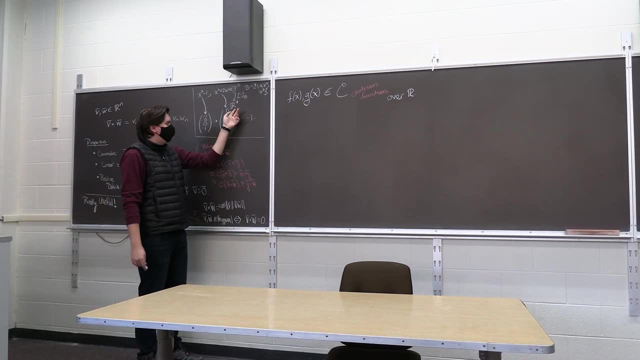 Like what's going to be our notion here. that would be analogous to dot product, Because we can't map this down into some nice rn- You know, r4, r10, or whatever- Because this is infinite dimensional. There's a lot. 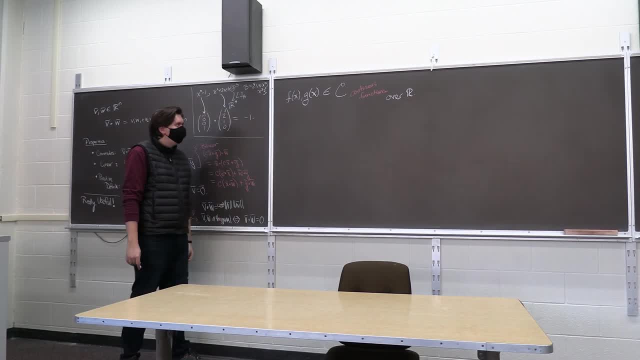 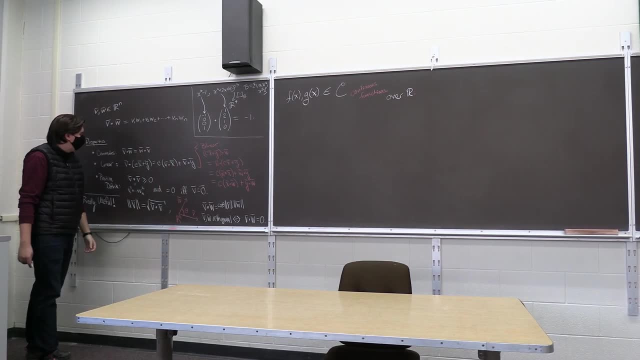 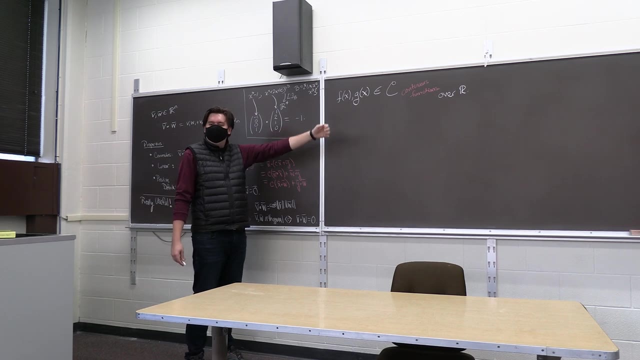 of continuous functions. right, It's really big. So what we want to do is we want to ask ourselves: well, can we come up with something that has these same kinds of properties for, say, continuous functions? So let's try and think. 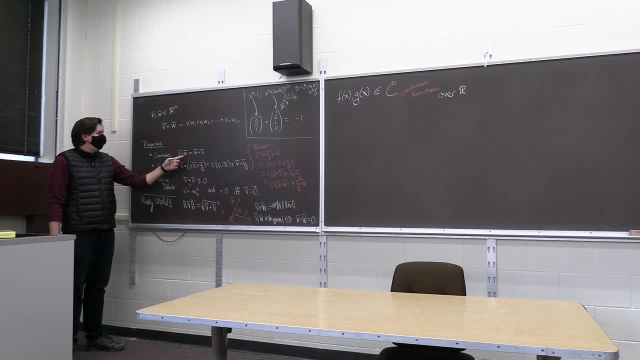 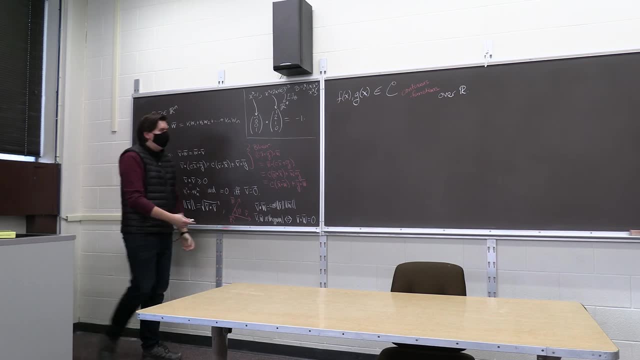 I have two continuous functions. I want a way of combining them that's commutative. I want to do something to f and g that commutes right. So I shouldn't take like f minus g. You know that's not commutative. 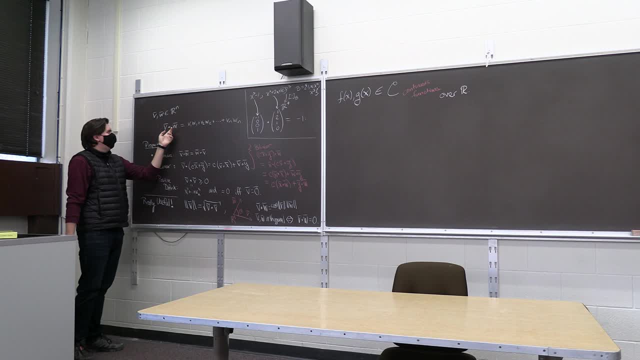 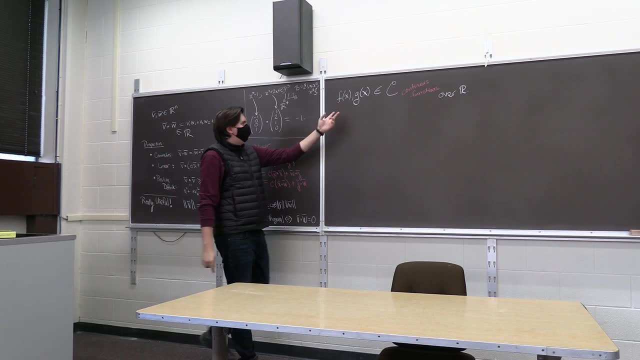 Also, I wanted to spit out a real value. right, Like, maybe the first thing I should have said about this is: the dot product gives you out a scalar. So I want one way of taking these functions spits out a scalar. I want it to be commutative. 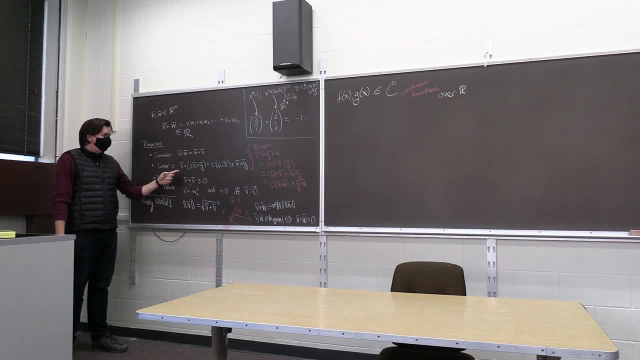 I want it to be linear, you know, Maybe just linear in the second term, but then with commutativity that'll give me its bilinear, And it should have this nice property of being positive definite. So it's like: what in the world can you do to functions? 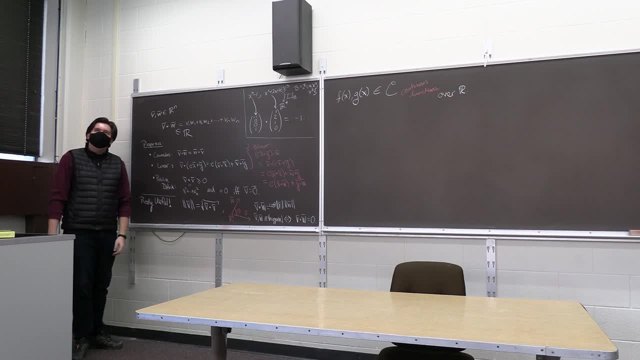 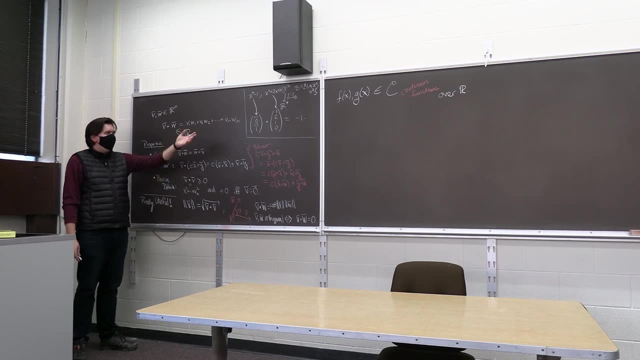 to do all these things. It's like, well, we could do like some kind of evaluation map and maybe that would give you the first two, Evaluate f and g, both at zero, and add those values up or something That would be commutative. 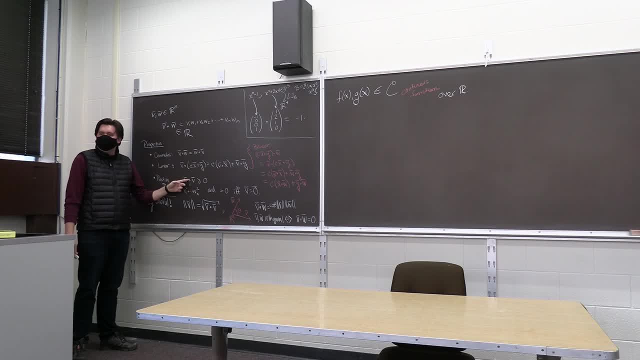 That would be linear, But it doesn't have this positive definite property. If you evaluate a function at zero, it's not necessarily going to be positive, right, It could come out to be some negative number. So like what could you possibly? 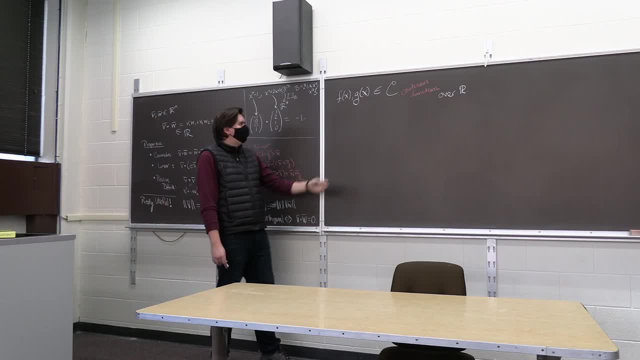 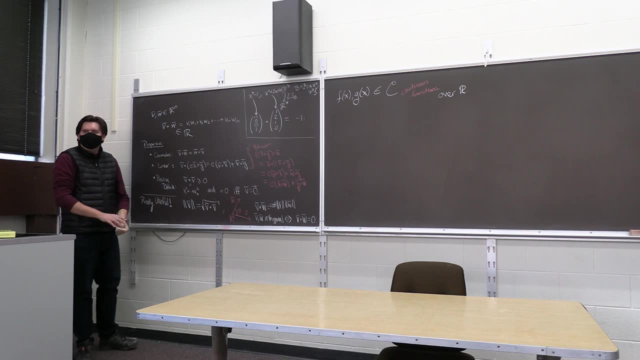 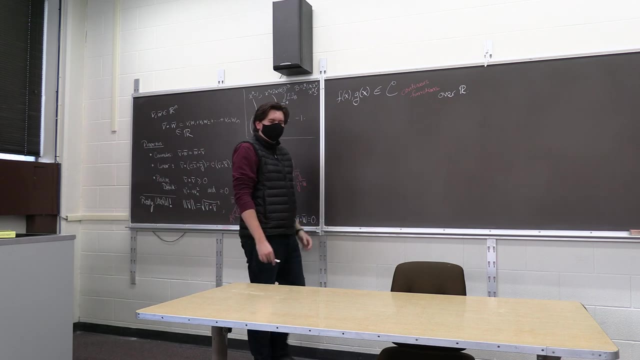 do to functions that will satisfy these properties? Well, do you guys have any guesses? Evaluation map doesn't seem like a good one. We're not going to just evaluate them at some number. That doesn't work. What else could you do to some functions? 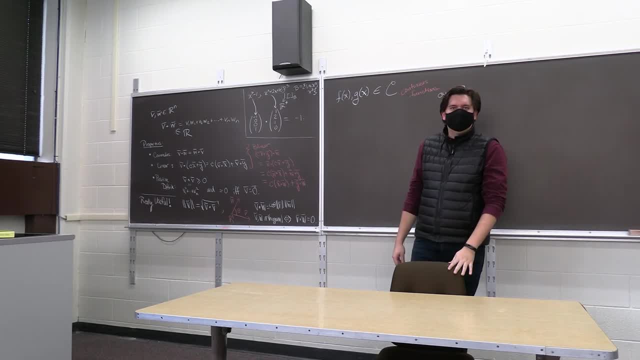 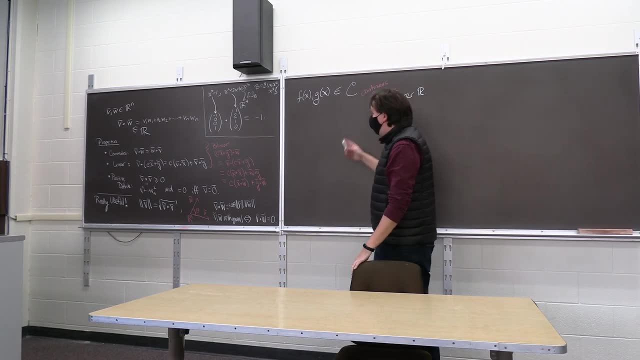 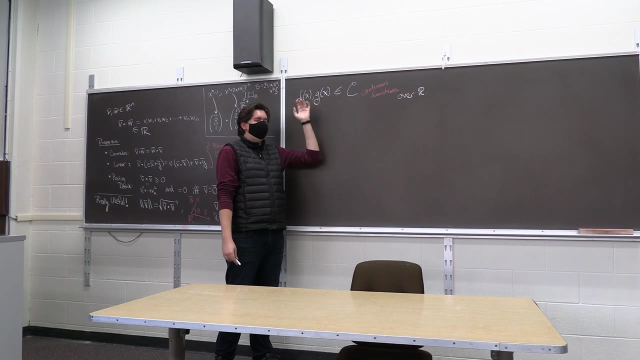 Continuous functions, Nice functions, Just guess things. Take a derivative. Well, no, because I want it to come out to be a real valued thing. right, It's like: well, take the derivative and plug in some value. like plug in x equals zero. 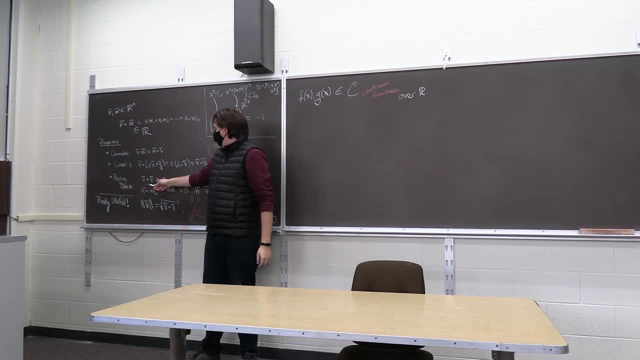 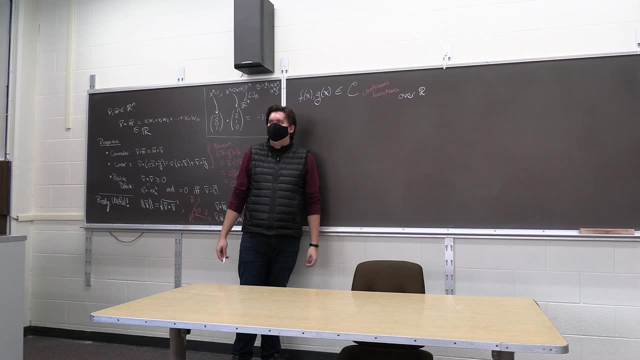 Yeah, well, I run into the problem here where this, may not you know something, dot itself would not be non-negative. So, any other thoughts? Any other thoughts? Well, let me give you one, Let me give you one. 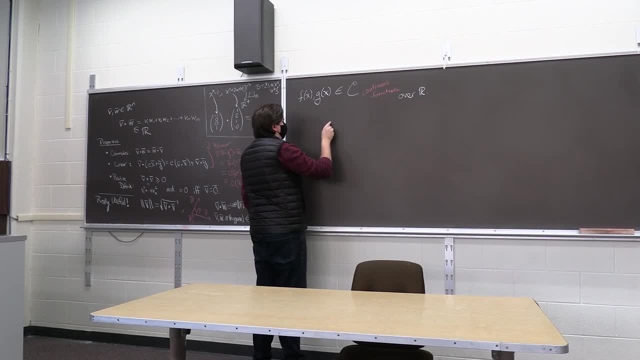 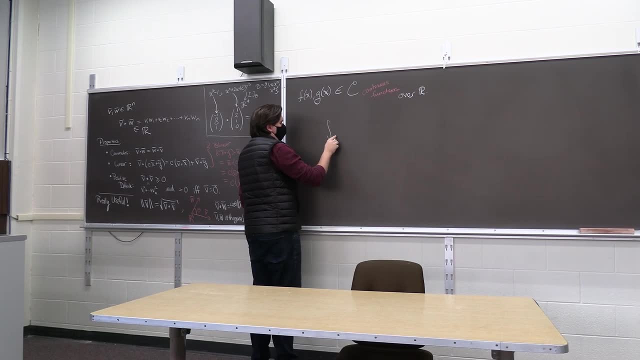 What we're going to do is we're going to take the entire derivative from. I need to pick, I need to make some choice From some a to some b. We could do from zero to one. I don't care. Whatever values you want. 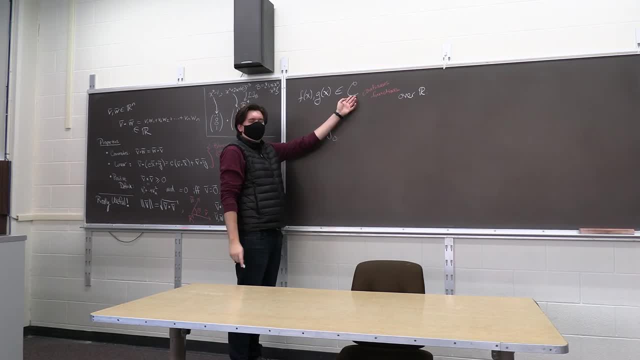 Let's do zero to one. Zero to one as long as it's continuous there. So if these are functions that are continuous everywhere, it's continuous from zero to one. If it's only continuous somewhere else, you know, just pick wherever it's continuous. 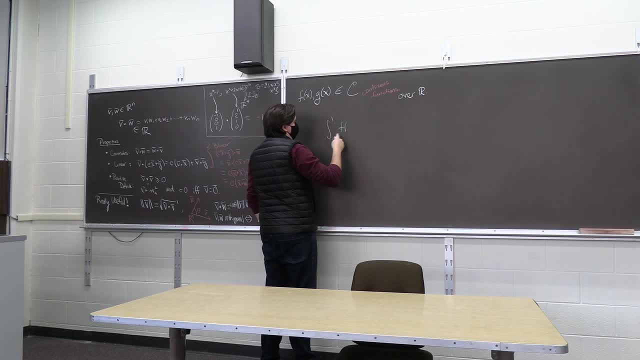 Pick an interval where it's continuous, Find the entire derivative of the definite integral of f of x times g of x- dx. I claim this satisfies all my properties, So let's check really fast. Well, first of all, what kind of thing does this spit out? 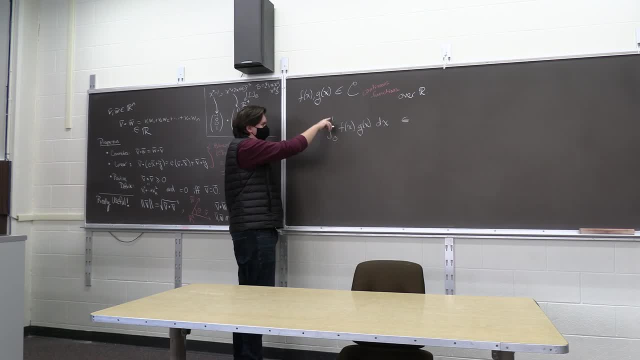 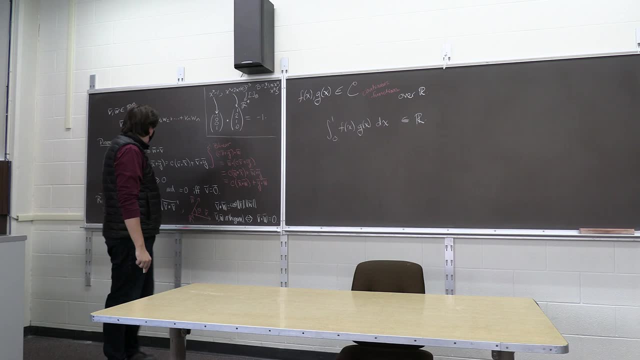 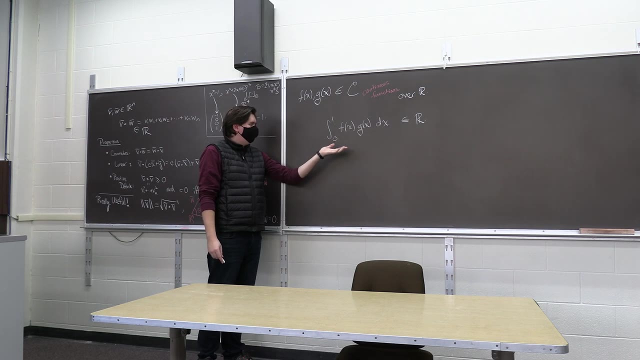 A real number? Yeah, Because it's a definite integral, So we'll end up with some value. that's real, So that's nice. How about this one? Is it commutative? Does this commute? Well, like, obviously. 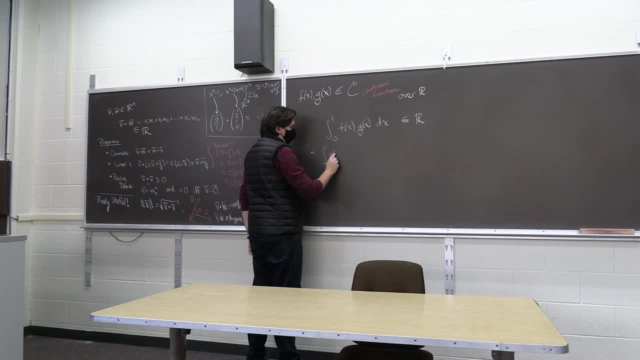 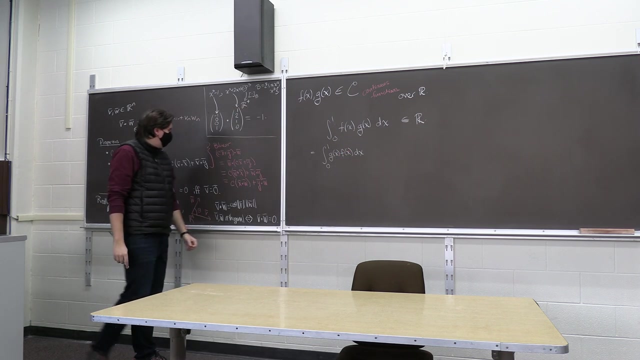 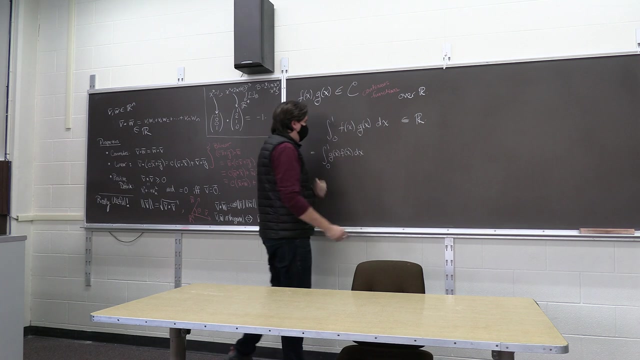 This is the same thing as just g of x times f of x, and calculate its definite integral from zero to one. because continuous functions commute, because real numbers commute, So it commutes. That's fine. Is it linear? It's like what is. 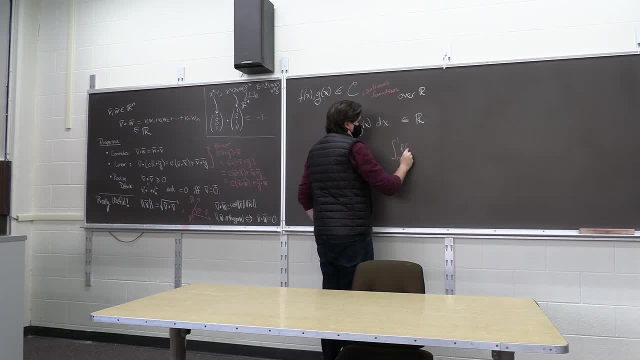 f of x times. well, let's try it, Some scalar times. well, I guess we could write it as like g of x plus h of x. So here I'm trying to see if it's linear. in the second argument It's like: well, 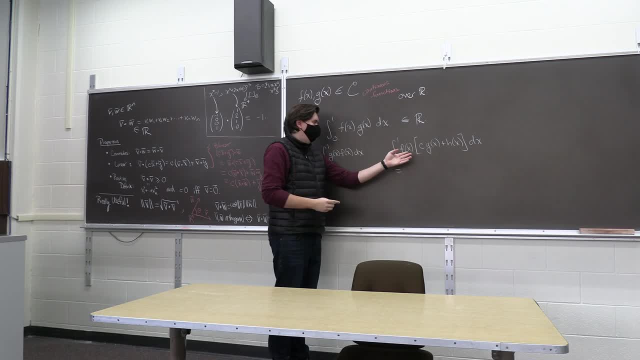 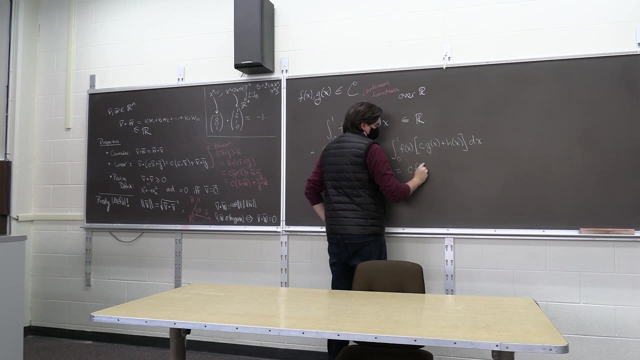 this just comes out to be: the inside is linear, right? Multiplication is linear because this is a real value function. So it's going to come out to be: since real numbers are, since multiplication is linear, this is just c, f of x. 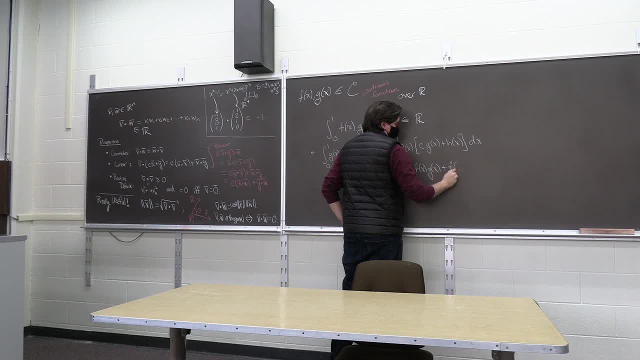 g of x, Just distribute Plus f of x, h of x, So like that's good so far, And then we just use the properties of definite integrals. It's like the definite integral of a sum is just the sum of definite integrals. 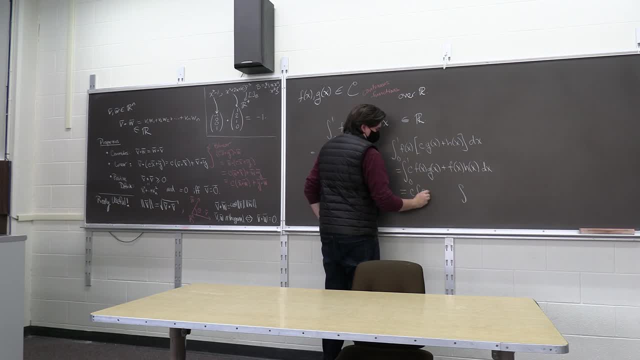 And when you have a scalar inside, you can pull it out. I think we talked about this before. an example like this. Well, I've made this same point. So, like that's good Linear, Well, it's linear in the second argument. 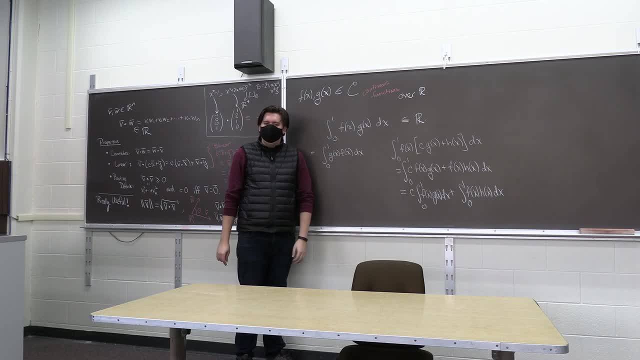 and it's commutative, therefore it's bilinear. Last thing is: let's check, if it's positive definite, What would be the integral from like 0 to 1 of f of x? now it's like v dot itself f of x times f of x, That's f of x squared. 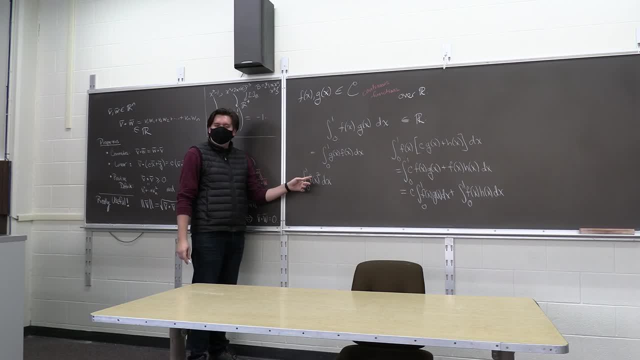 Ah Well, f of x squared is a non-negative function, right? You add up its area from 0 to 1, so that will come out to be some non-negative value. And then my question is: when is it 0? Why? 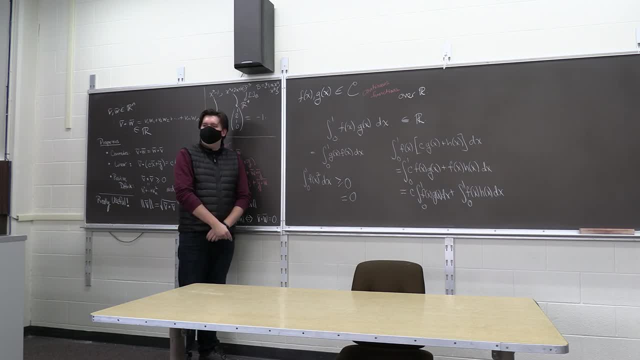 Because it's a positive real value or positive continuous value function, then whenever you take the integral anywhere, it's not 0. It'll arrive at some area, Alex. Well, the example that came to mind is if we take a continuous function- negative x, from negative infinity to 0. 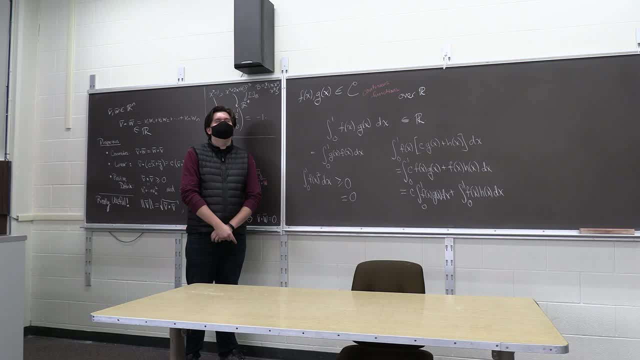 and then have it be 0 from so a piecewise function. it'll still be continuous, but have it be negative x from negative infinity to 0. have it be 0 from 0 to 1 and then have it be x minus 1 from 1 to infinity. 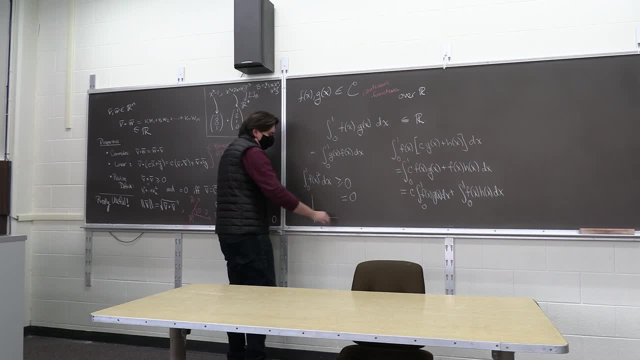 Oh, oh oh. You're saying that it has to be exactly 0 on the interval from 0 to 1, but outside of that interval it could be other values. True, Okay, So it has to be exactly 0. this will only come out to be 0. 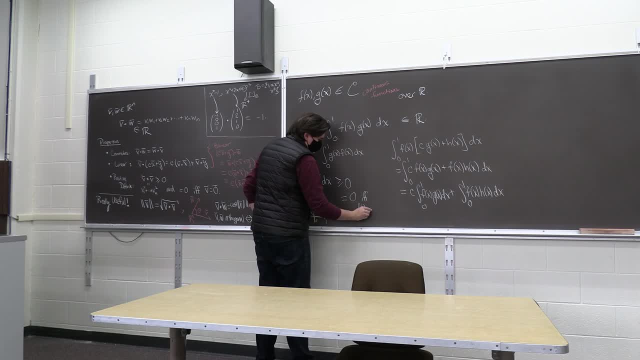 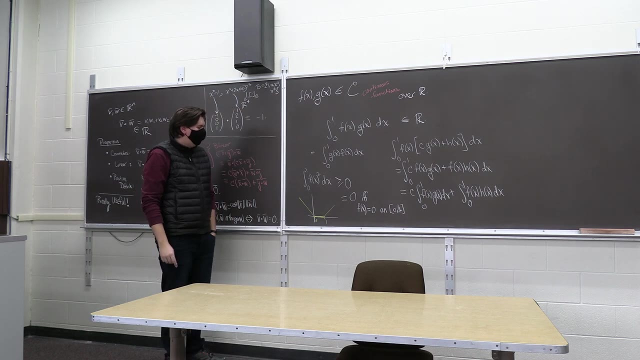 if, and only if, your f of x is identically 0 on. you know, here it's 0, 1 and in general it's going to be whatever a and b you pick, whatever interval a and b, that's a good point. but the point is here: between 0 and 1. 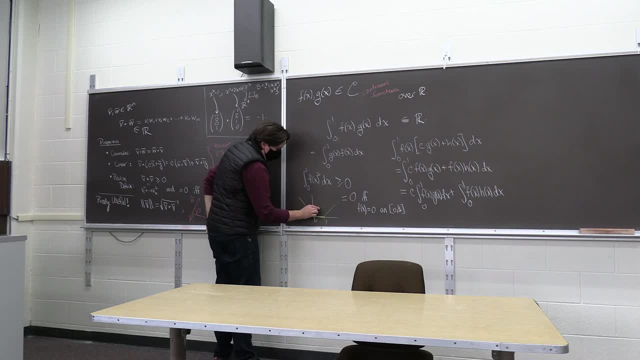 it has to be identically 0, because if you had one point that was not 0, by continuity, close by points would also be non-zero. right, I can go down really fast, but as long as you're if you've done any kind of real analysis. 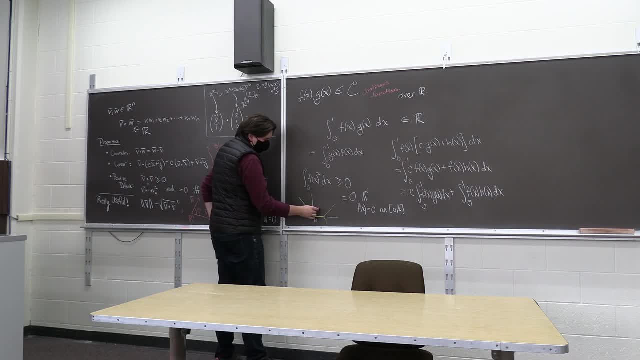 or if you know the epsilon delta definition of continuity. it's like you can't just have one point here and then suddenly jump to 0 everywhere else. that wouldn't be continuous. so for this to be continuous it must have like a whole little section here. I mean you can go down really rapidly. 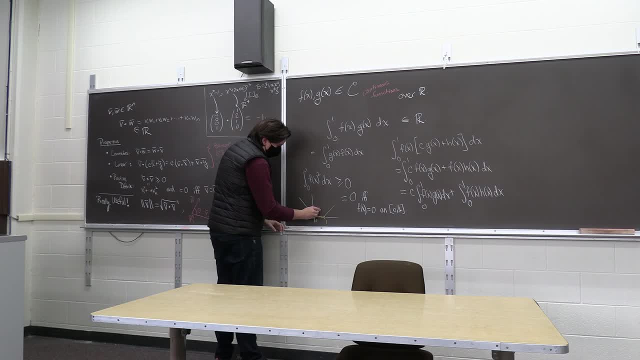 but it must have a whole little section. and then you're like: well, that has some non-zero area, right? so it has to be identically 0. it has to be identically 0 because it's continuous, at least on that interval. good, okay, so if you'll grant. 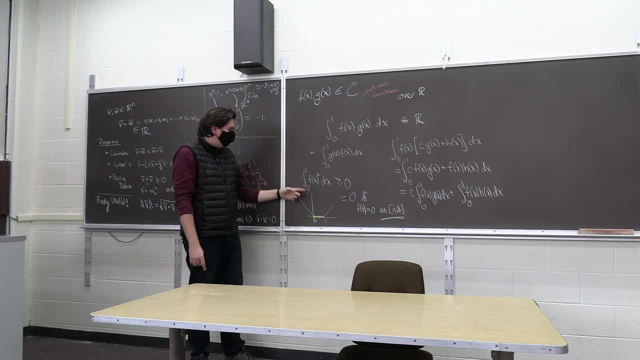 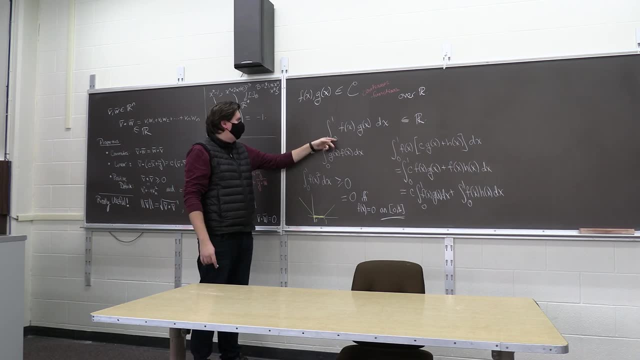 that I mean you can just say: we're just thinking about these functions restricted to the domain 0,, 1 or whatever. if you want to do some other domain- 0 to 10- you can just do that definition instead. okay, so this works. 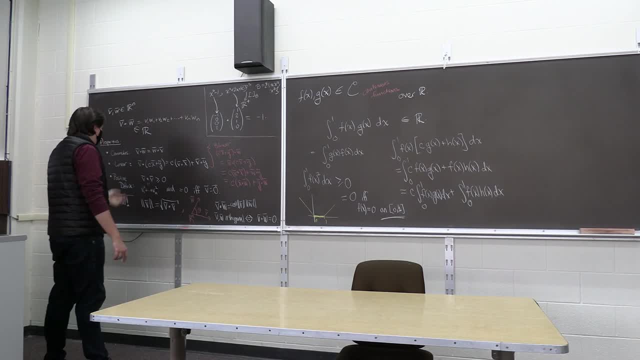 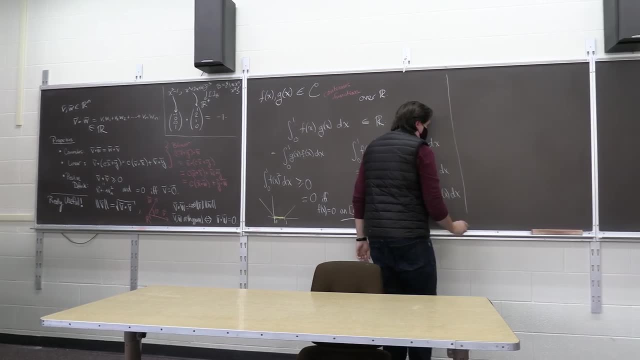 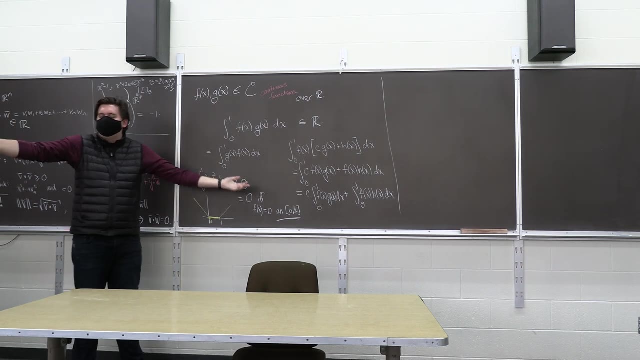 this works. this gives us the properties we care about. well, should we try one more? I mean, there's other vector spaces we've seen. what if, instead of having your vectors be functions, they could? what else? what other kinds of vectors we've seen not like? 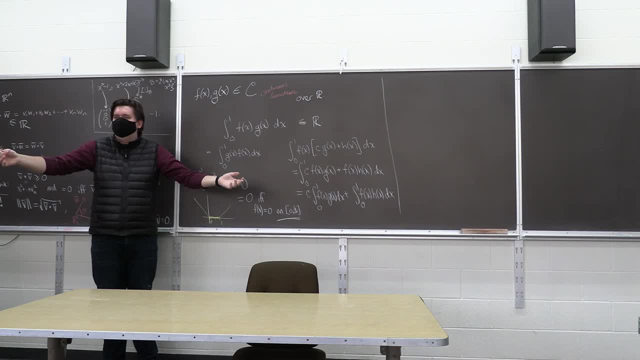 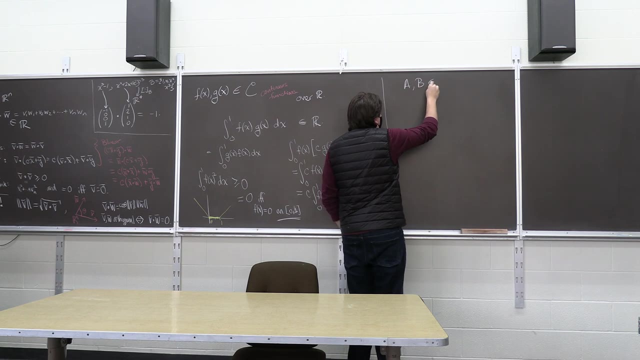 things in our n, not like just functions, what else? what's another vector, space? we've talked about matrices. so let's say you have two vectors, where your vectors? now I'm going to call them a and b, and let's make them matrices. let's make them m by n. 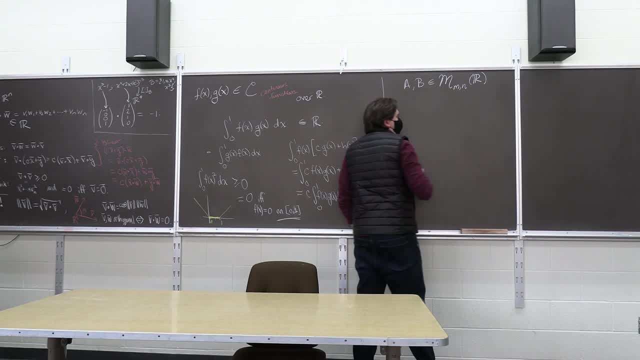 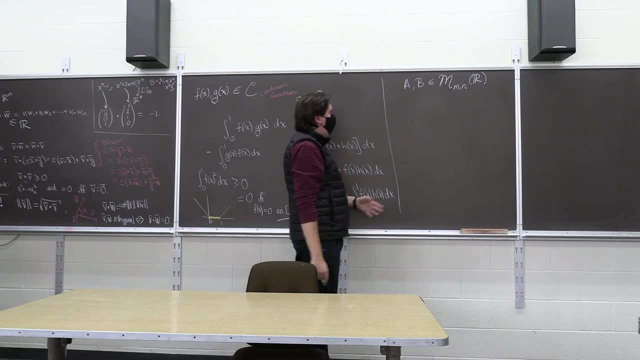 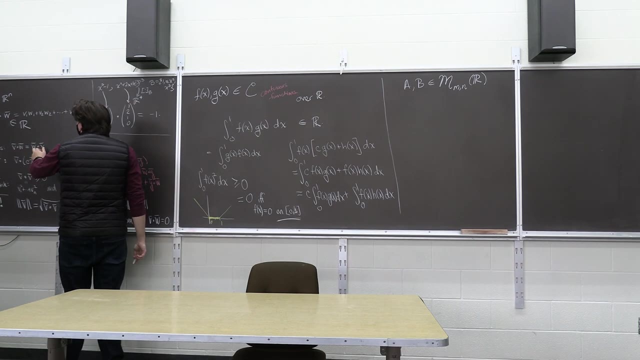 matrices and for simplicity, we'll just keep them to be real valued. it's like: okay, now what can I do to these matrices? well, there's a lot I want to do. it should be some operation that commutes. it should be linear. it's bilinear, it should be. 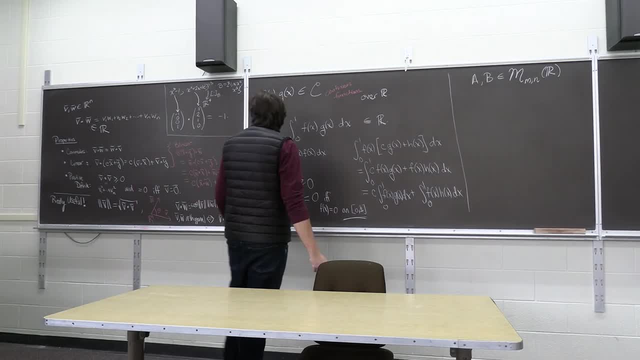 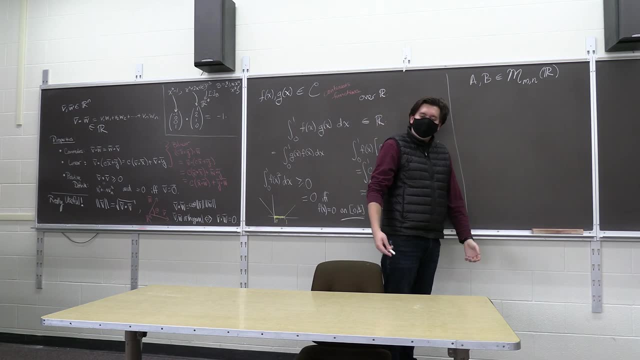 positive, definite. how are we going to do this? and I want to come up with a real number. and how do I take two matrices and end up with a real number? well, first of all, you have a problem where it's like these matrices are very different sizes. I mean, well, they're the same. 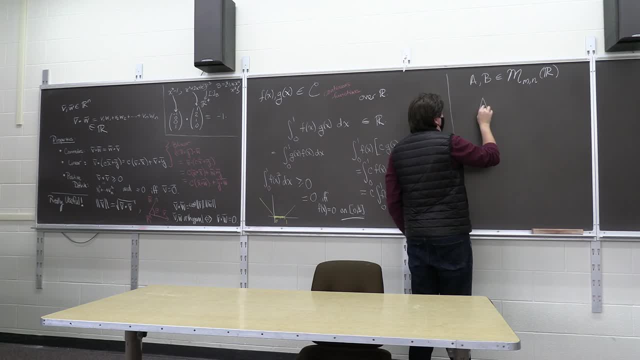 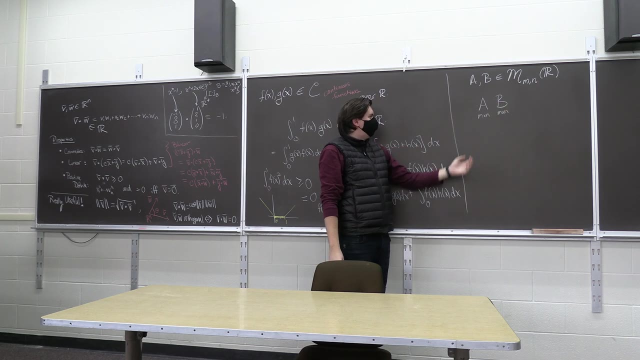 size. but it's like because they're the same size you can't just do like a times b, because you have like an m by n times an m by n, so already it's like that's not defined. like what could I do so I could multiply them? 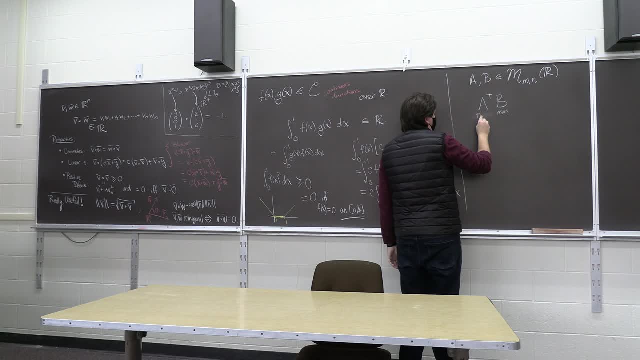 yeah, if you transpose one of them. well, now it's an n by m, so at least the multiplication here is defined. but the problem is, we now end up with an n by n matrix. I don't want to end up with an m by n matrix, I want to end up with a number. 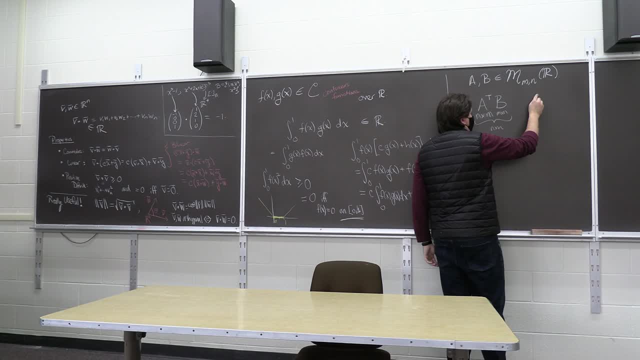 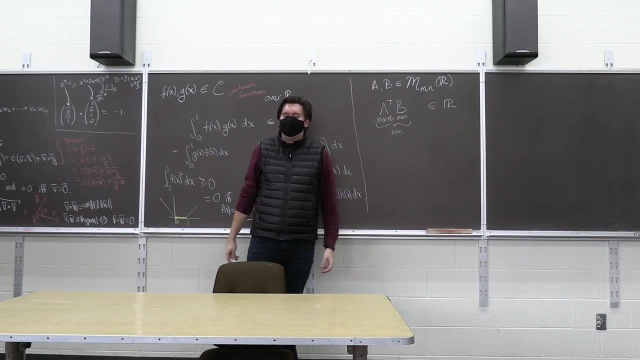 a real number. so what do I need to do to this to make it turn into just a real number? how do you turn a matrix into a number? what's some function on a matrix that spits out a number? determinants are a great idea, but here's the problem. 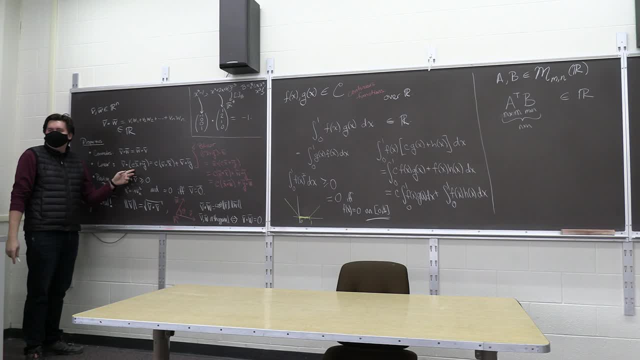 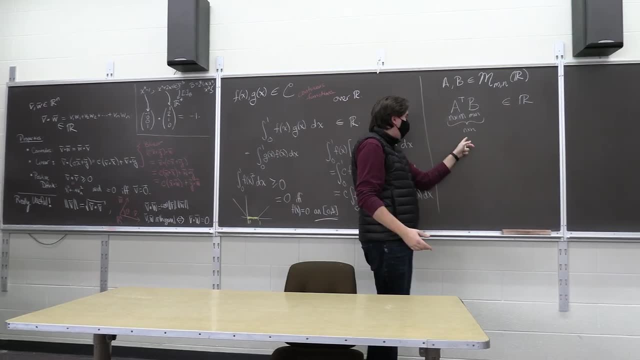 is the determinant linear? we talked about this before. no, so linearity is going to fail if you use determinants. so what's another function that eats in some matrix and spits out a square matrix? now, eats in a square matrix and spits out a number. 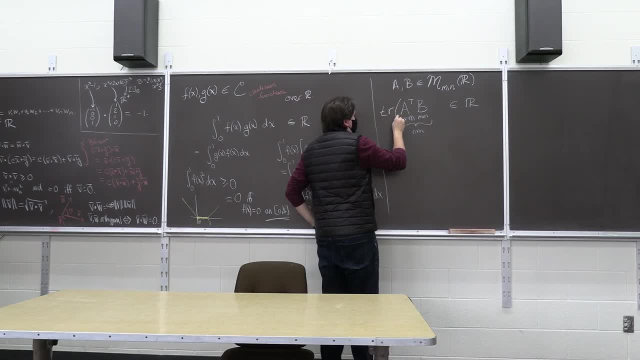 trace. let's try that. let's try and define it this way, ok, well, first let's check: is it a commutative? so you know it's like. so we have the trace of A transpose B, and over here I have the trace of B transpose A. 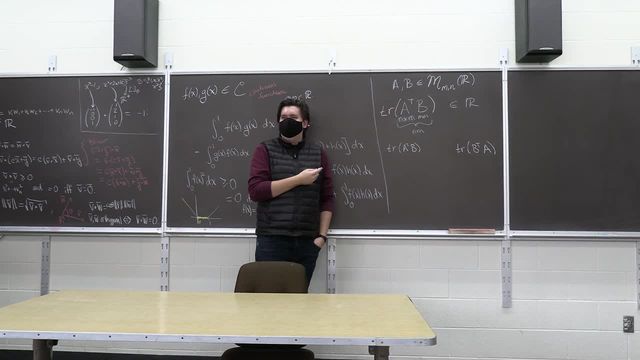 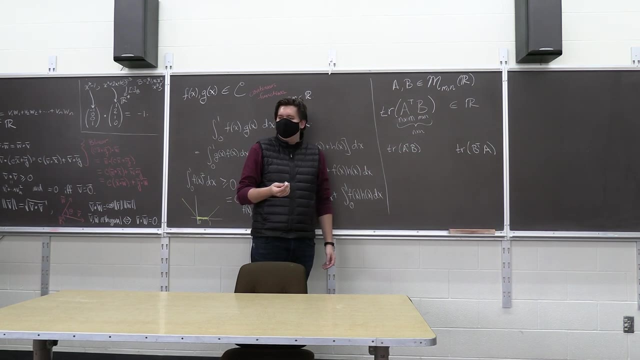 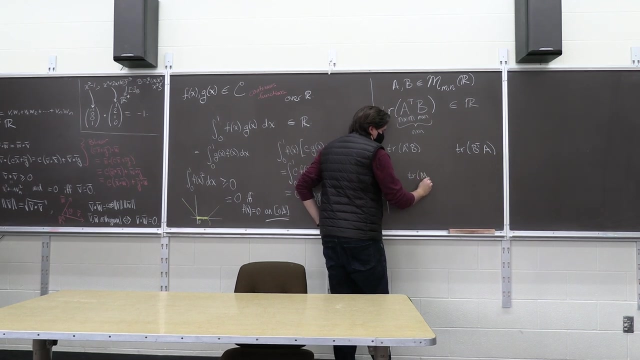 so is it the same thing? why, or why not? are they the same? what property makes these the same? yeah well, there's something you do to a matrix that keeps the diagonal the same. let's take in the transpose in general, if you have some matrix and you take its transpose. 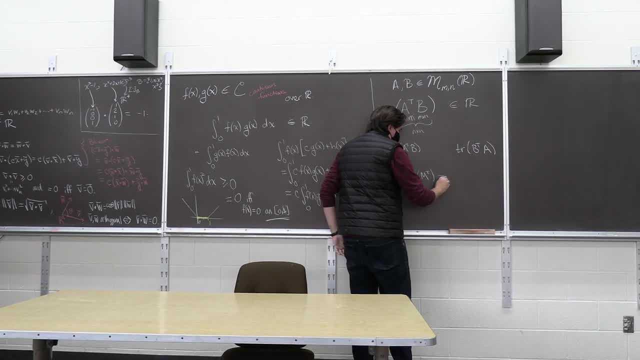 the diagonal stays the same right, and so the trace of the transpose of a matrix is the same as the trace of just a matrix, which means the trace of A transpose B is the same as the trace of A transpose, B transpose. but what is A transpose, B transpose? 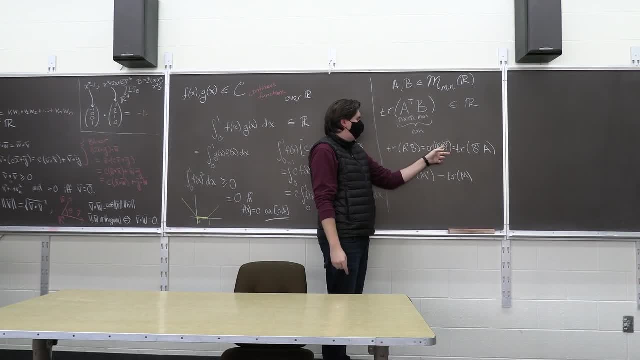 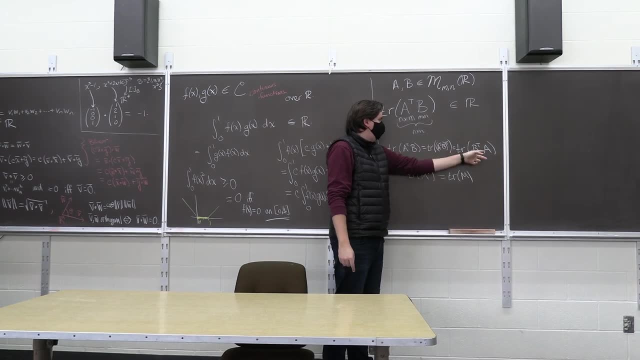 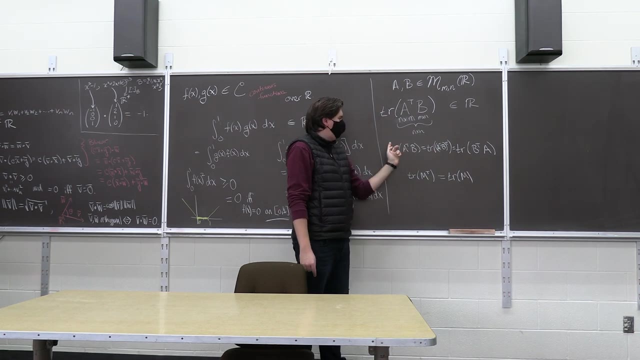 well, now you have to remind yourself the way you do a transpose of a product of matrices is you do first the transpose of the second, then times the transpose of the first. A transpose, transpose is A right. so here we're using a couple properties of transpose. the diagonal stays. 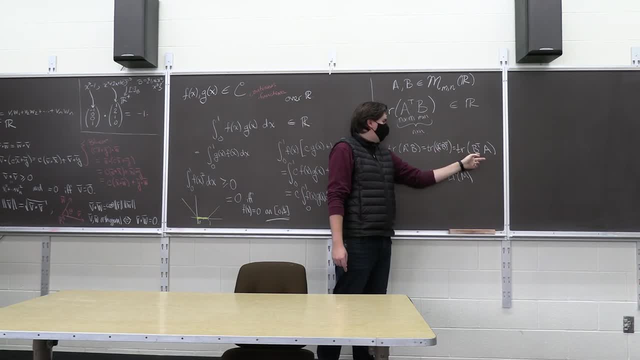 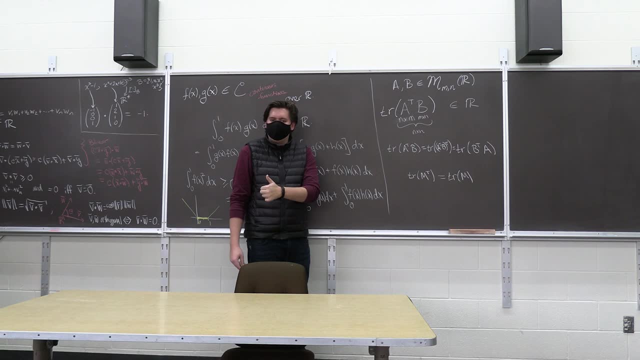 the same and the transpose of a product is you reverse the order B, transpose times A. ok, so like: yes, it's commutative, so this is pretty promising. is it linear? well, we kind of designed it to be linear. the trace is defined to be linear, so you can check really fast. 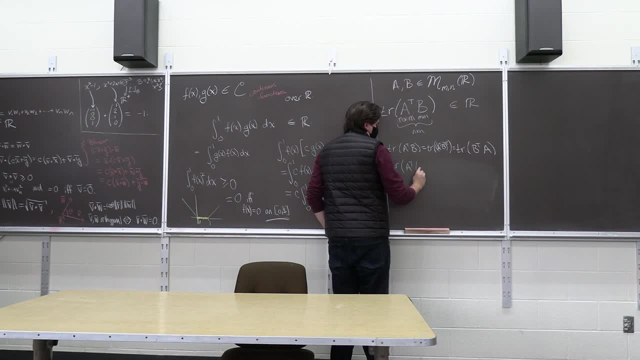 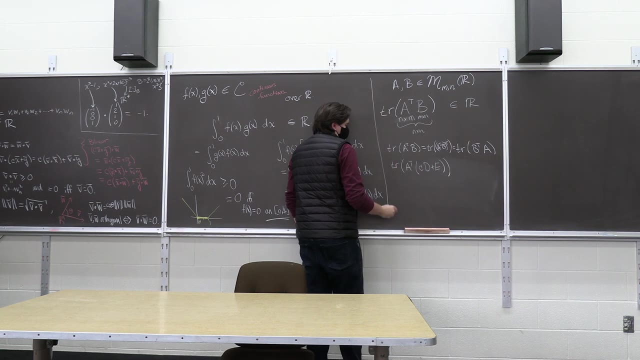 what is the trace of A transpose times, some scalar copy of I don't know the matrix? uh, if I use a big C you might get confused. let me just say D plus E, it's like. well, distribute this and you can pull out the scalar. so that's just the. 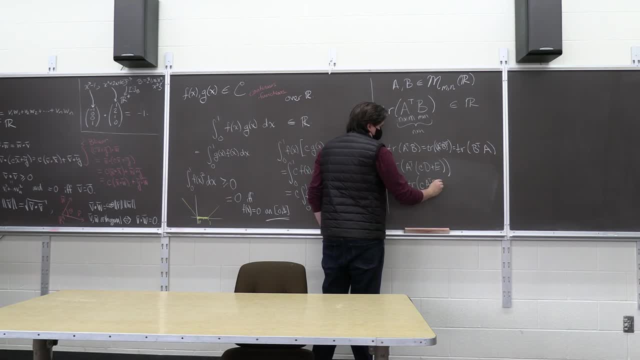 trace of your scalar of A transpose D plus A transpose E. and we picked trace because trace is a linear operation. this is just the trace of C, A transpose D, plus the trace of A transpose E, and then it's like: ok, it's a trace of some. 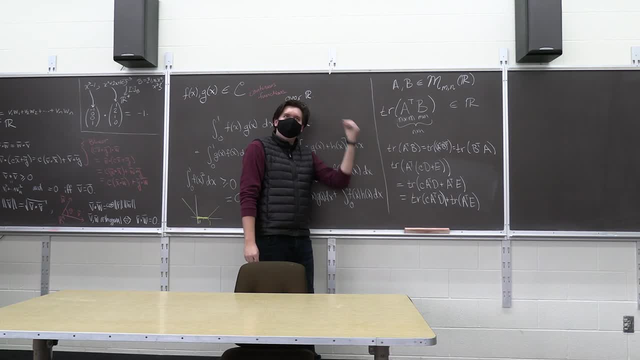 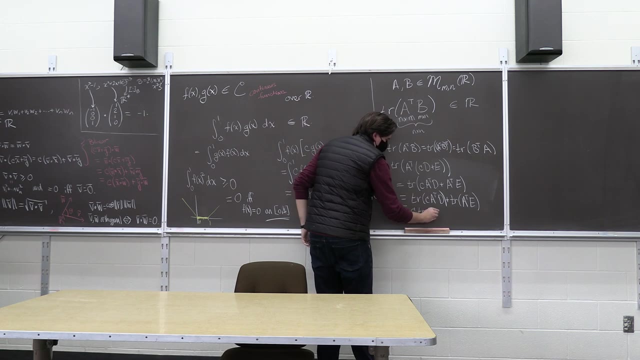 scalar times a matrix. if you're scaling a matrix, you're scaling everything on the diagonal by C, so it's the sum of all these things scaled by C. so I can factor out the C and I get C times the trace of A. transpose D plus the trace. 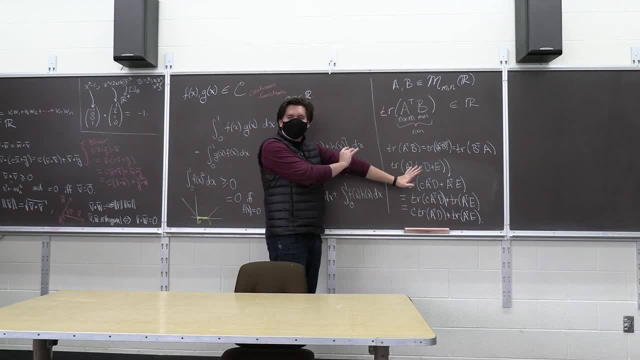 of A, transpose E. ok, it's linear, linear in the second argument, but then, because of the commutivity, it's bilinear. what else do we want to check? positive definite. now this one. this one might seem like a little bit more challenging. like what is the trace of some? 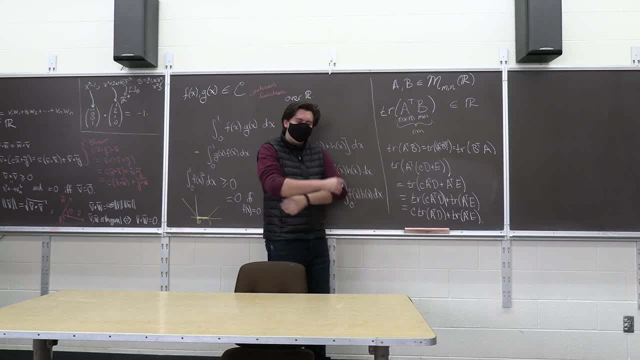 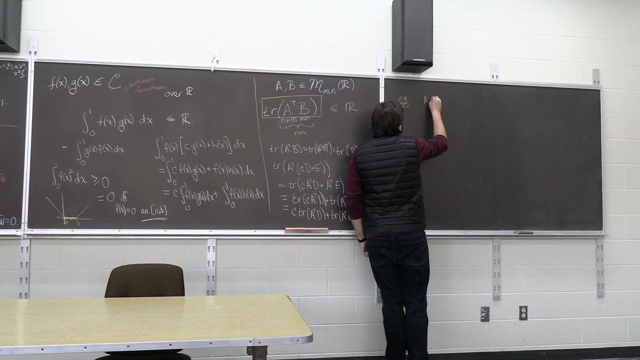 A transpose times itself A. it's like huh, that one might throw you off. but here's a trick to help you see it. let's just think about what this guy actually is like. what is this? let's look at an example. let's say: A is some matrix. 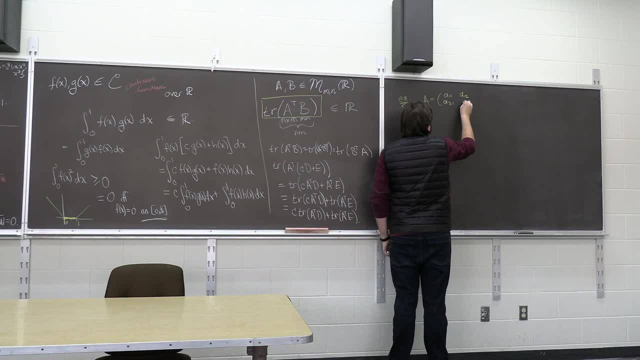 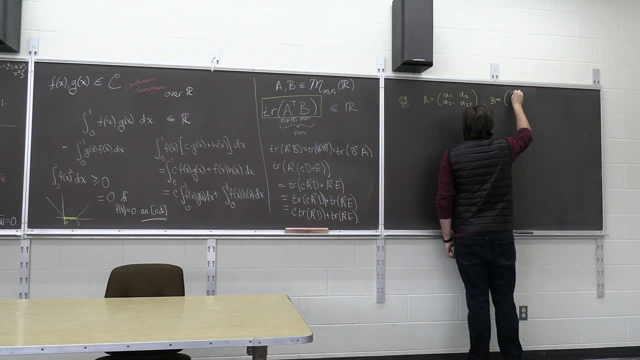 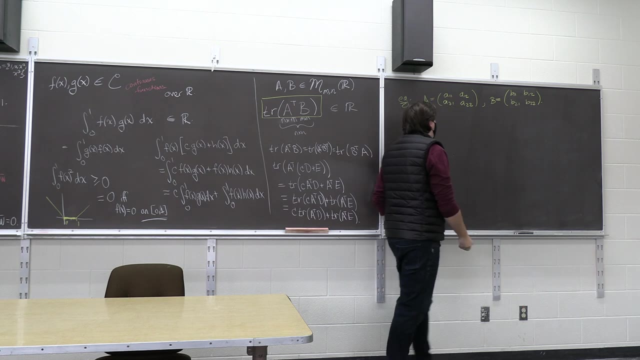 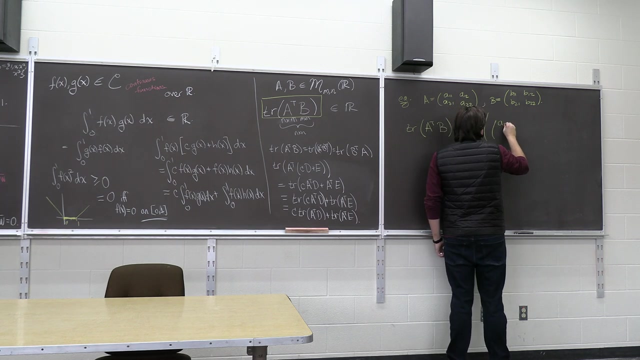 A11, A12, A21, A22 and B is some matrix: B11, B12, A21, B22, then A transpose times B. taking the trace of that is taking the trace of this. transpose so A11 down, A12, A21 and below it, A22. 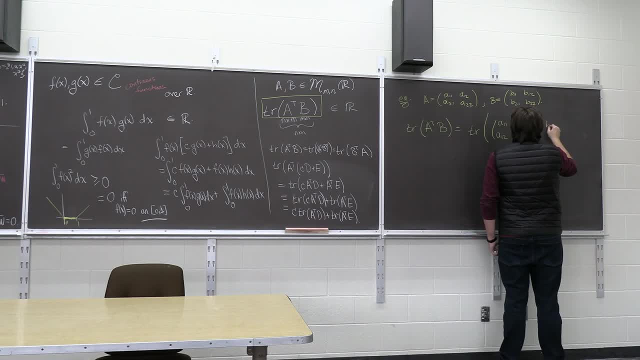 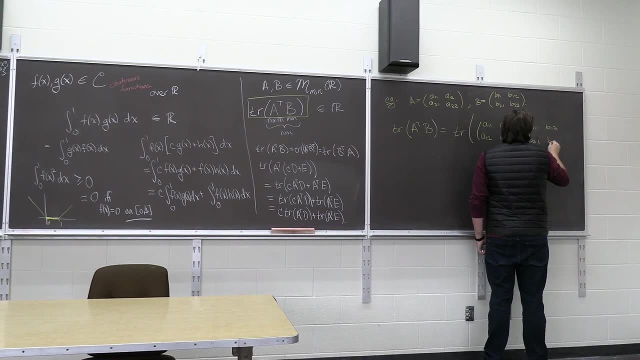 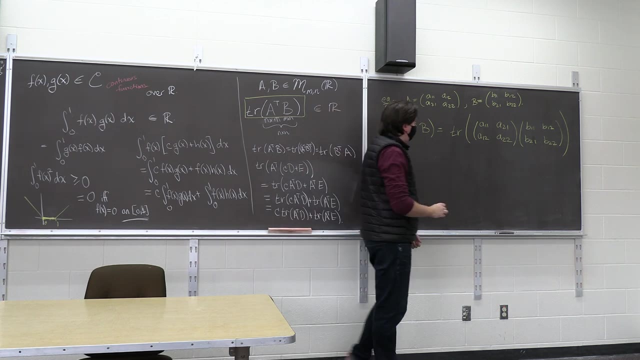 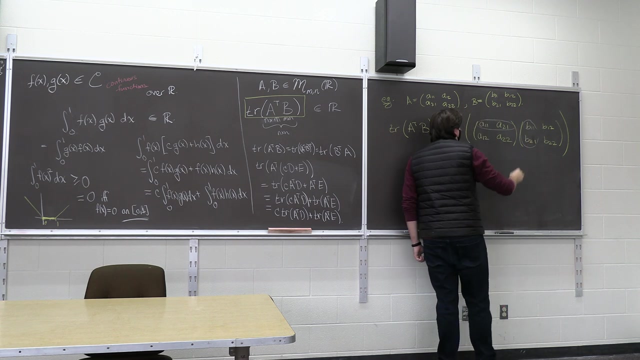 took the transpose of the first one times the second: B11, B12, B21, B22- and let's think about how this works. matrix multiplication is going to be row times column. that will give me the top left value of this matrix. and then I want to know what the bottom right. 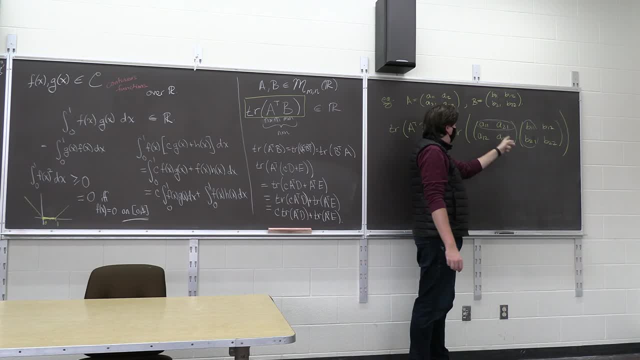 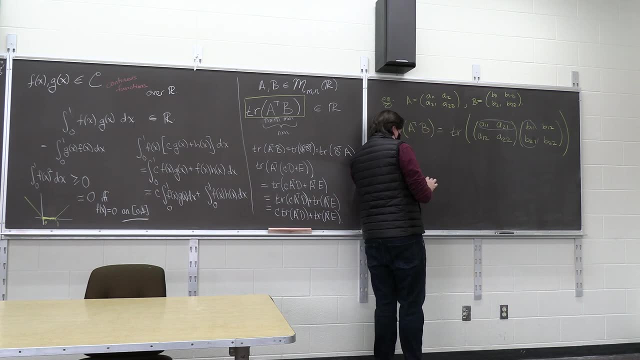 value is because the trace is adding up the diagonal. so it's this first row times this first column. so the trace is going to begin with the top left element on the diagonal, which is just going to be A11, B11 plus A21, B21 plus that's the top left. 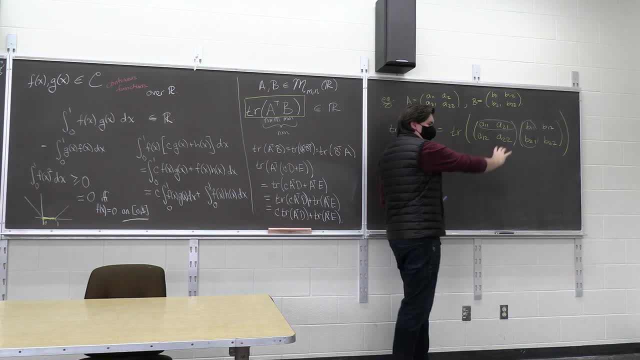 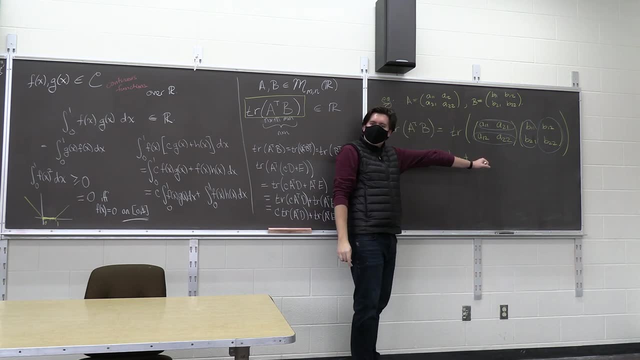 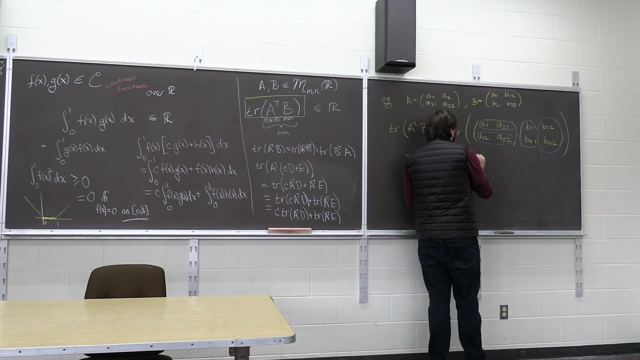 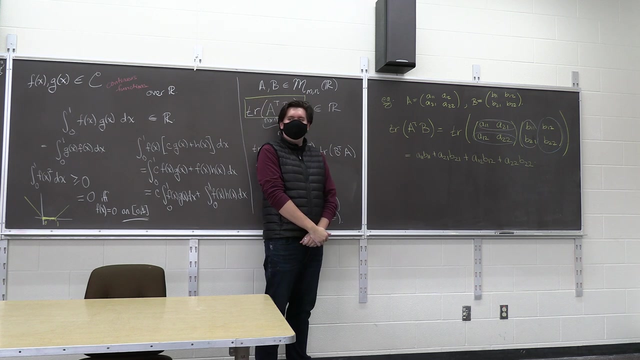 element and now I want to do to get the bottom right, the bottom times the right. that will give me my other diagonal value and notice how that comes out. that's just A12, B12 plus A22, B22 and in general, even if you don't have two by twos. 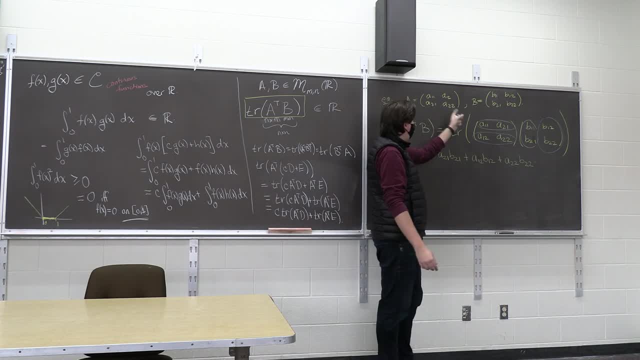 pick whatever size it's like, because you take the transpose of this one, it's now. it's like the row of the transpose would have been the column of the original, so it's like you're just going to be doing the first column times, the first column plus. 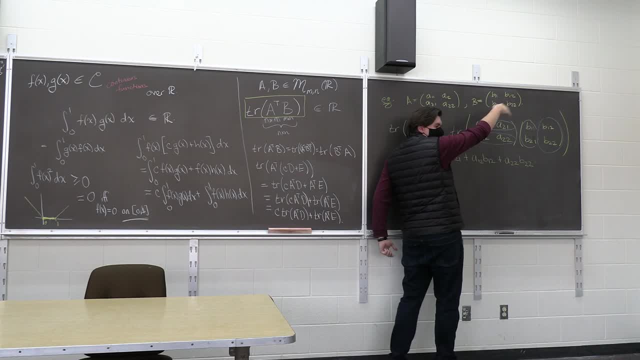 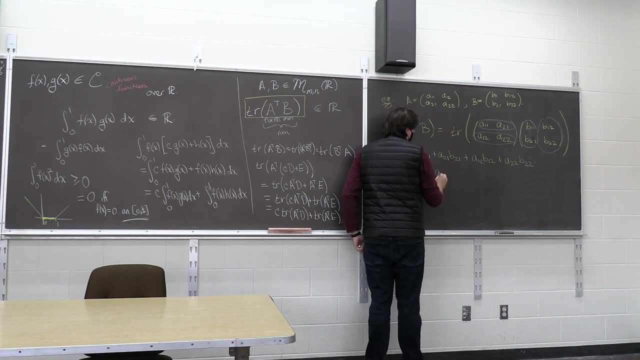 the second column times the second column plus the third column times the third column and so forth, which is exactly just going to give you the sum. of you know, A I, B, I A. I should say A I J, B I J. it's just the cross-bonding values. 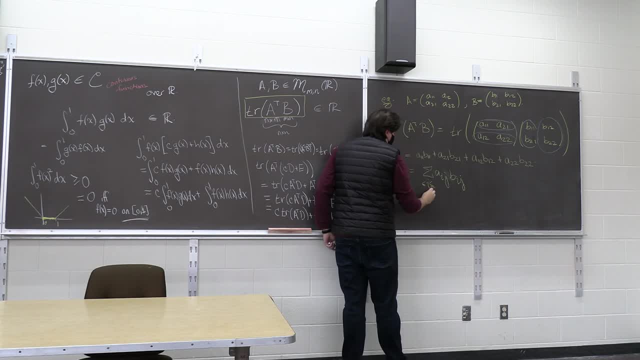 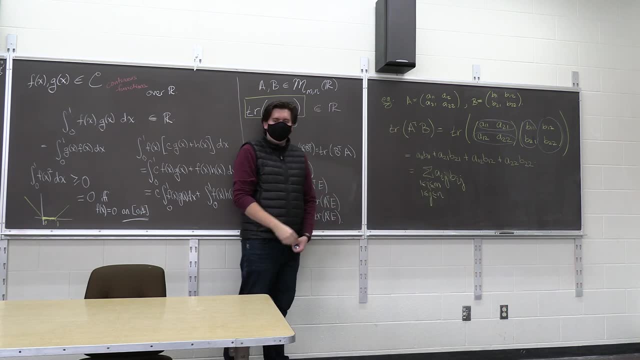 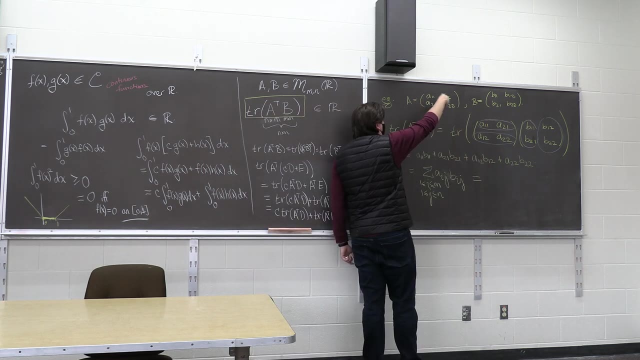 where your I is just varying over your rows and your J is just going over your columns 1 to M, 1 to N. that is, what is this operation really doing? well, it's like you're just thinking of this matrix as if it had just been a single vector. 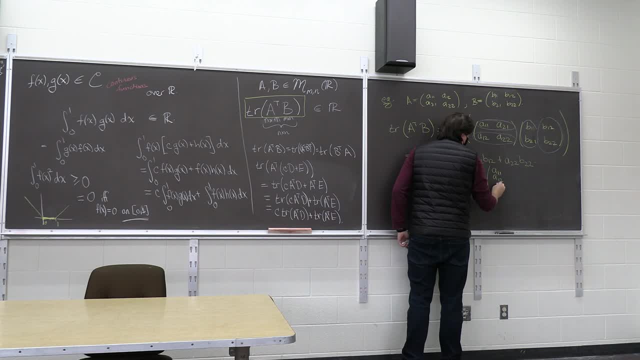 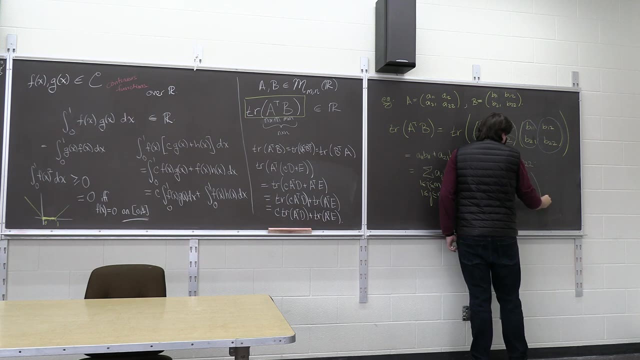 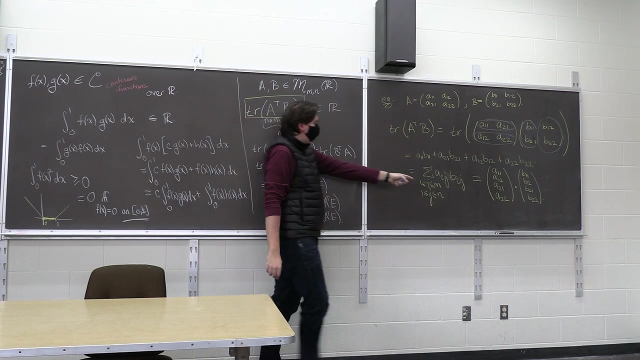 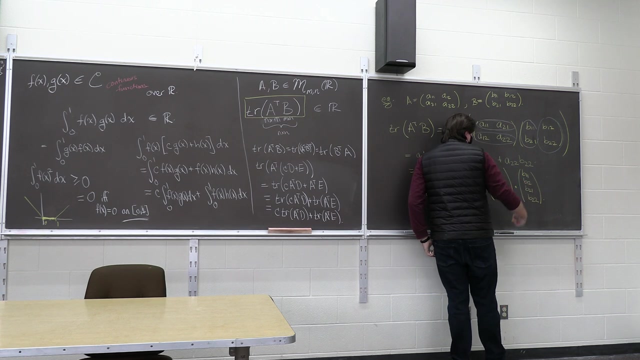 A11, A12, A21, A22 and dotting it with this other guy: B11, B12, B21, B22. right, you can think about this operation as being analogous to a dot product inside of some space. you know, these guys would live inside of R4 and R4. 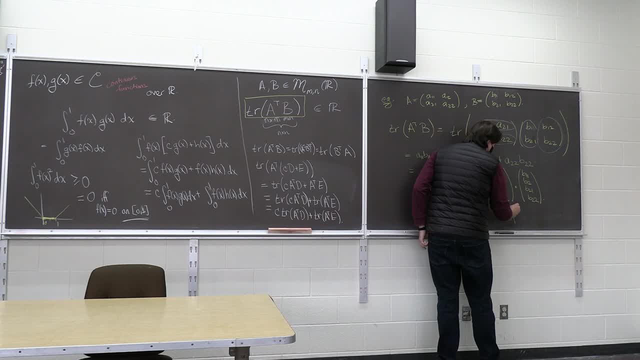 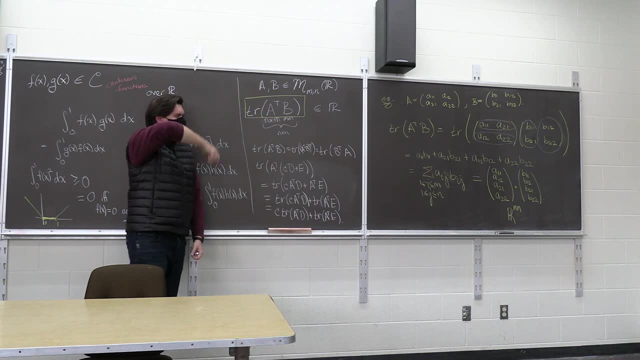 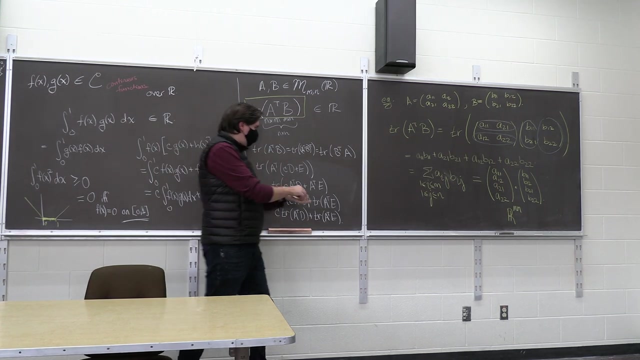 in general it lives inside of R M N because it's just all the values of your matrix lined up into a vector and then dot the other one. but we've already said the dot product satisfies these properties, so will this right? it's like: what is the trace? 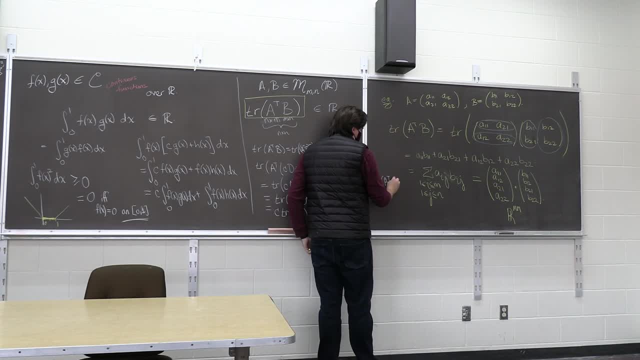 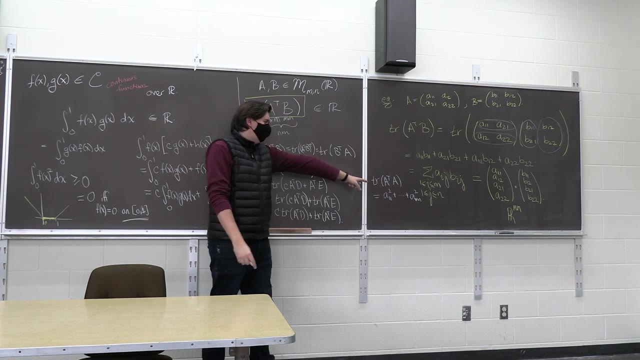 of some matrix, A transpose times itself. well, that's going to be A11 squared plus, you know, all the way up until the last entry of A, whatever A, M, N is squared. and then it's like: clearly, that's positive, definite, it's greater than or equal to zero and it's only zero. 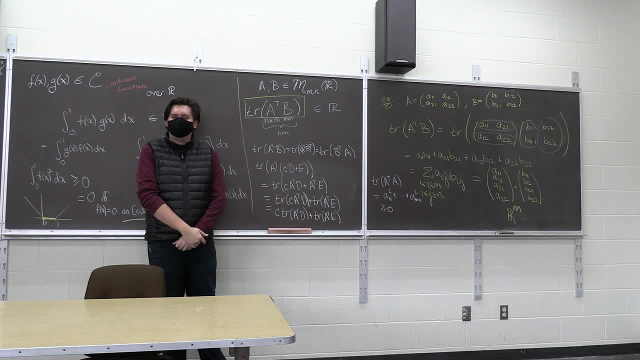 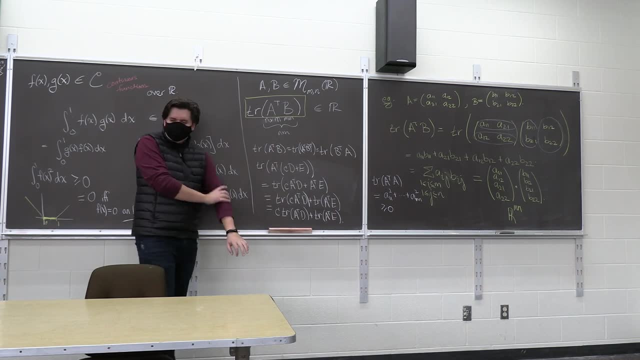 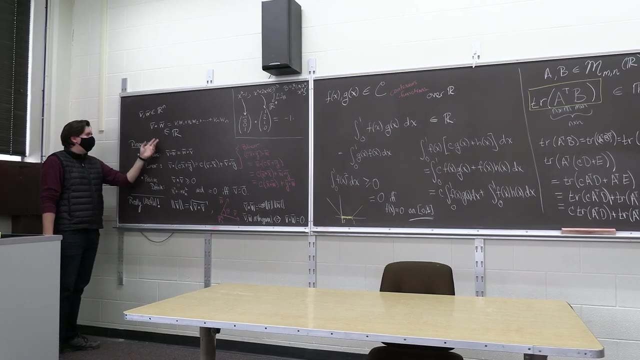 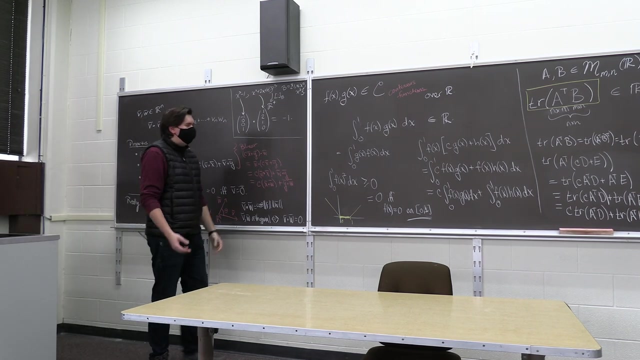 and all values are zero. okay, I've probably belabored the point a little bit too much, but here's what I've been wanting to say. we started out with a dot product. we said it has these three nice properties, and then we looked at other vector spaces. 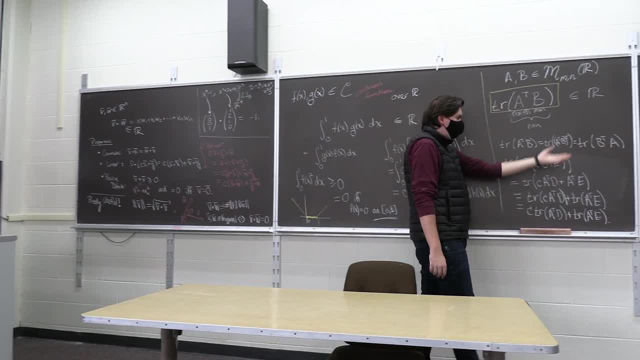 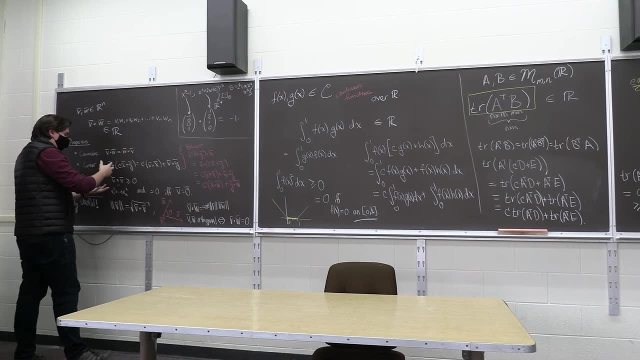 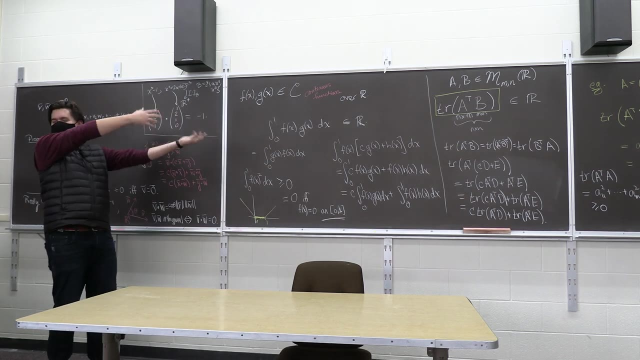 and we said: well, we can find functions that have the same properties, and so what we do in math is like: well, we really care about the dot product. it has these nice properties. there are other things that have the same nice properties, so let's give some name to all of these things. 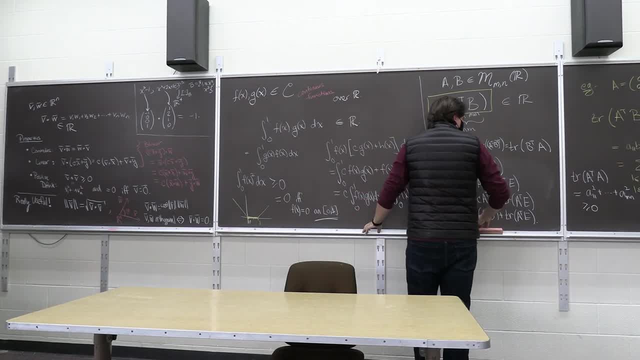 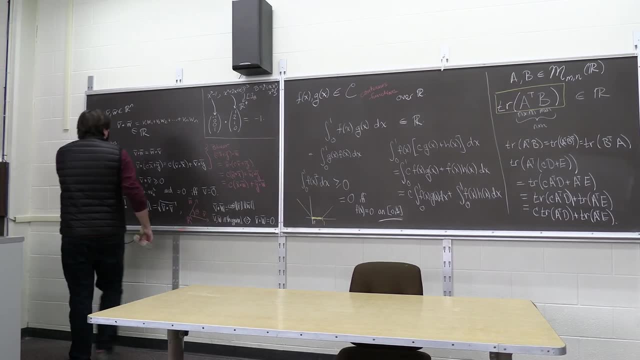 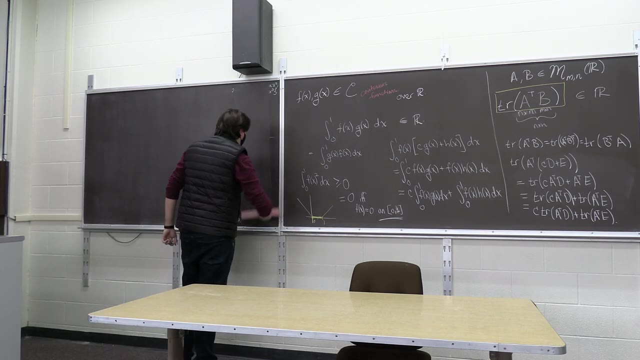 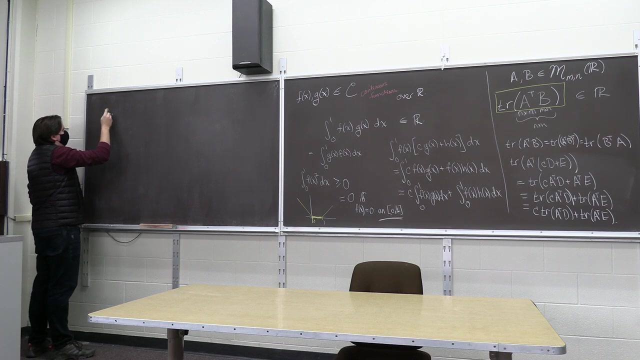 and so what we're going to call this is we're going to call this the inner product, so I'm going to have to erase this, but we remember what the properties are, so let's give it a name. so here's my definition. given some vector space, v. 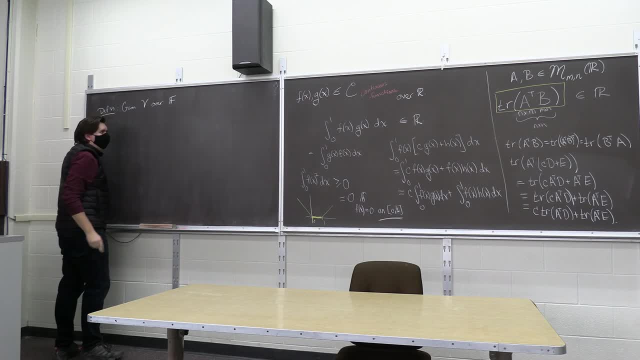 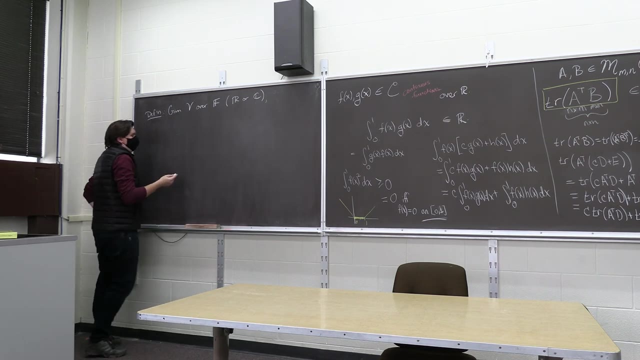 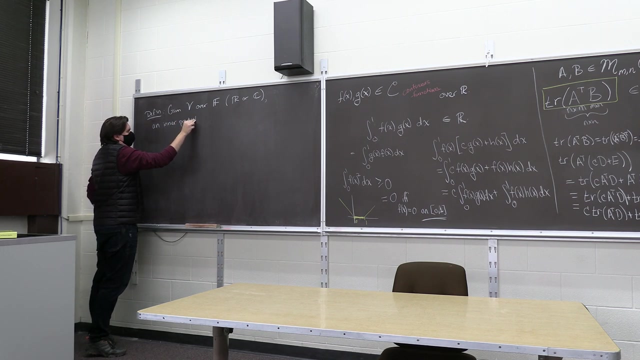 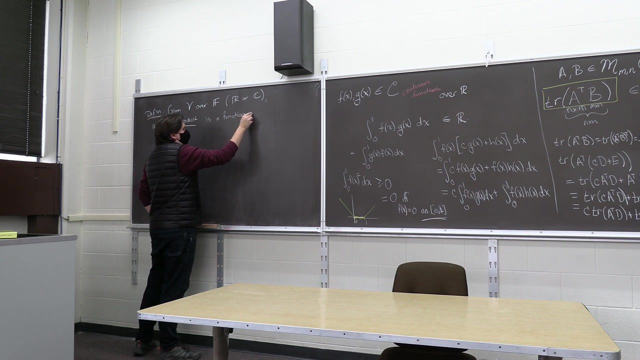 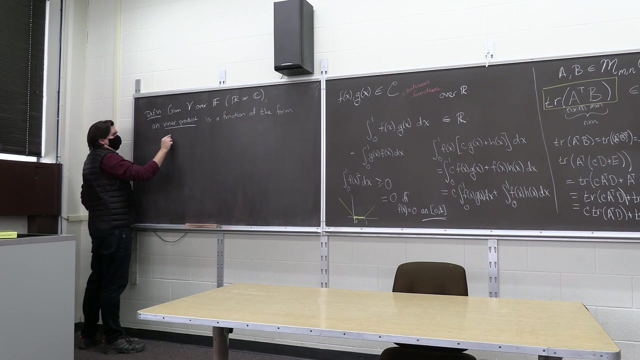 over a field and for us that field is going to be either the real numbers or the complex numbers, given some vector space over that field in inner product is a function of the form. it's going to take two vectors in v and spit out some scalar in your field. 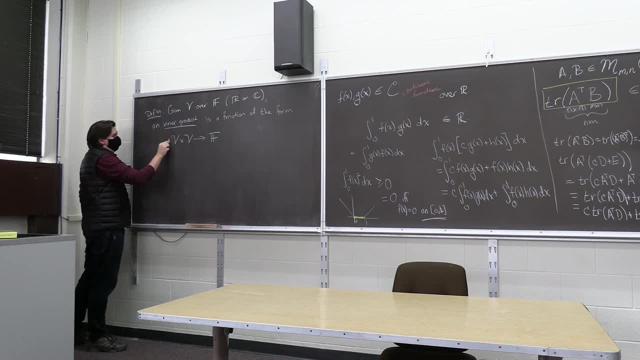 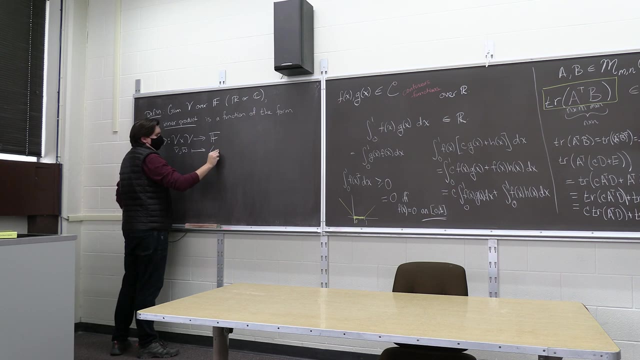 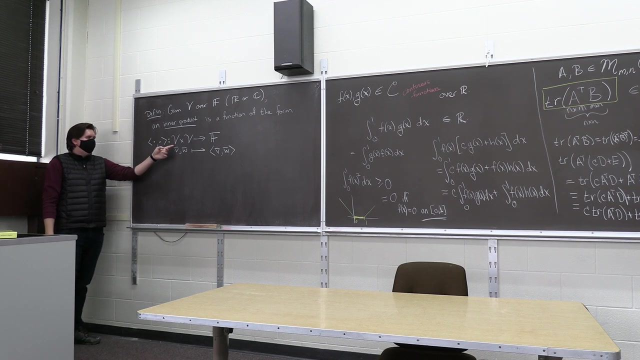 and the way we typically denote the inner product will be with these fancy brackets. that is, if you take some vector v and w, the inner product will be denoted with these fancy brackets. so it's a function that takes a vector in v and a vector of v. 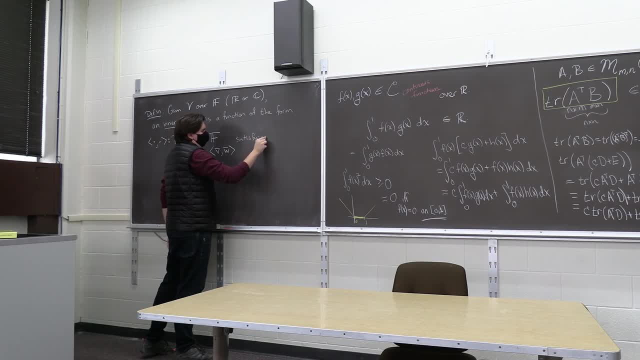 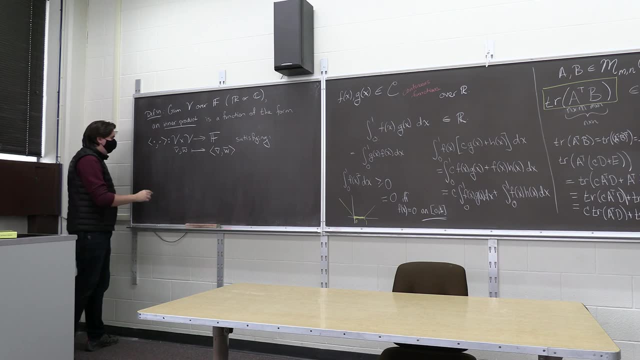 satisfying. I'm going to lie to you, but it's for your own good. it should be commutative. vw equals wv. it should be linear in one of the terms: v. okay, let's do some. multiple of x plus y should be. we're going to pull out. 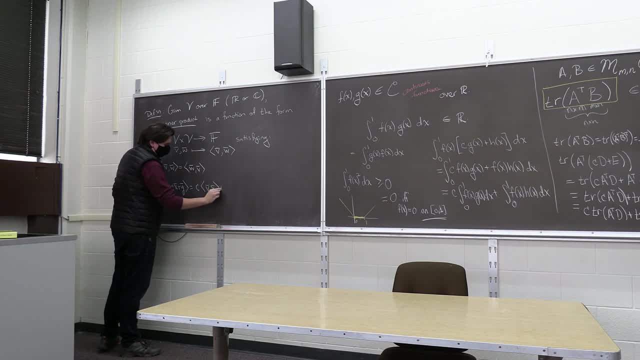 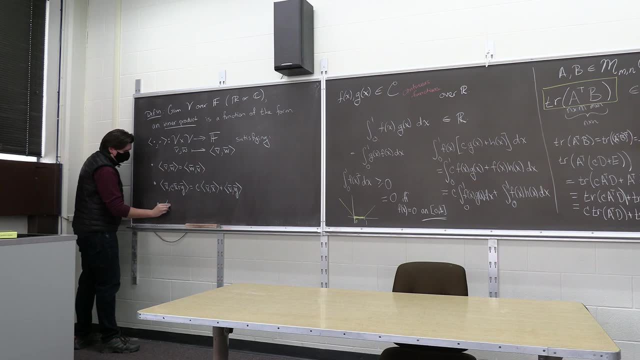 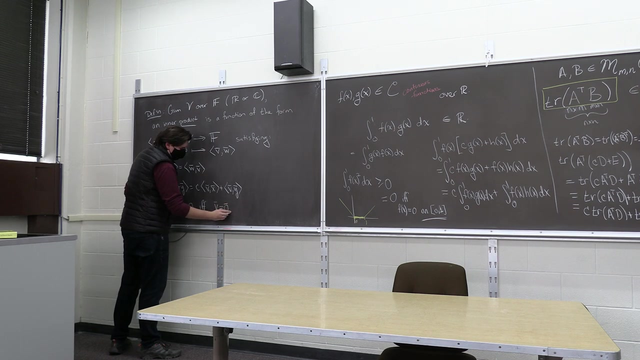 that scalar c, v's inner product with x, plus v's inner product with y, and it should have this property of being positive. definite vv, the inner product of v and v, gives you the scalar zero if, and only if, your v is identically zero. granted, we saw, 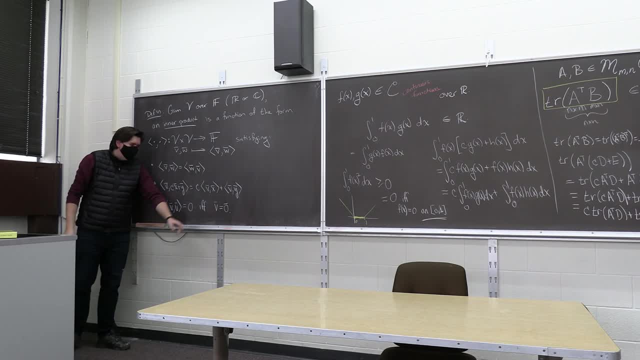 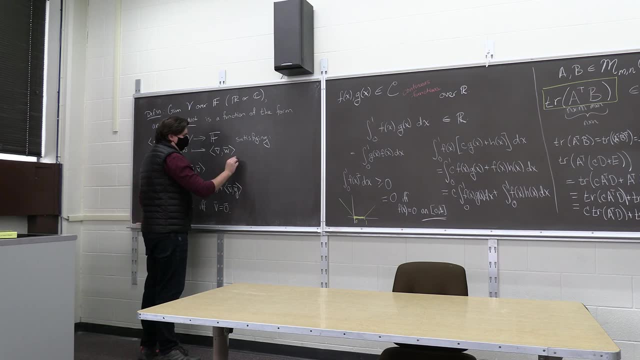 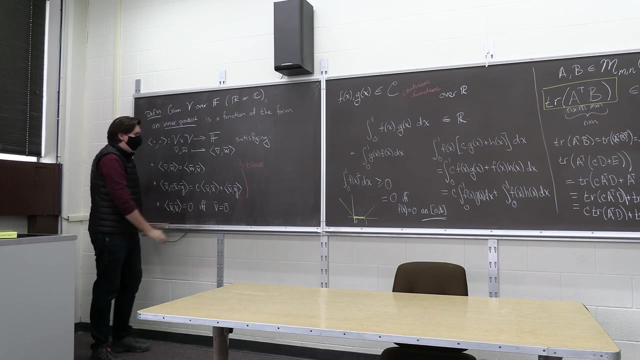 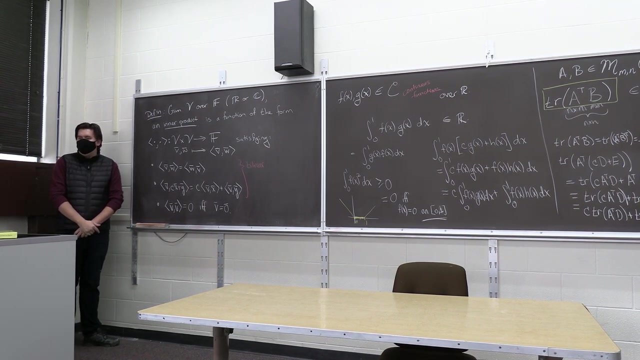 on some domain or whatever. we can be careful about what we mean by that, but that's the spirit and, just like before, these two properties together give you that in fact, it's a bilinear form. okay, I lied, this is almost true. this would be true if we're working over the reals. 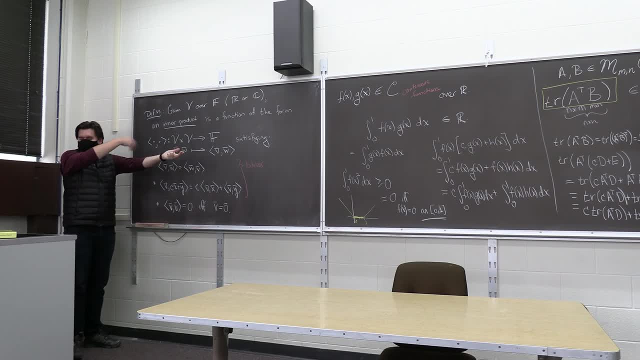 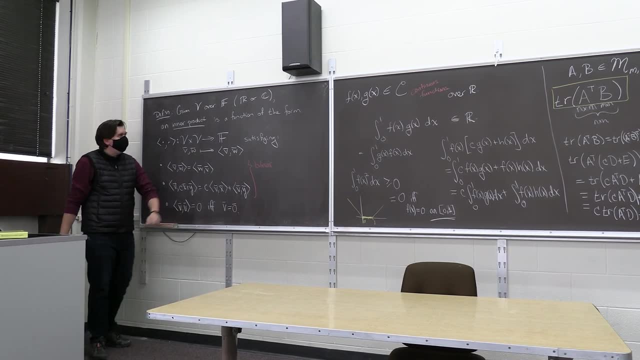 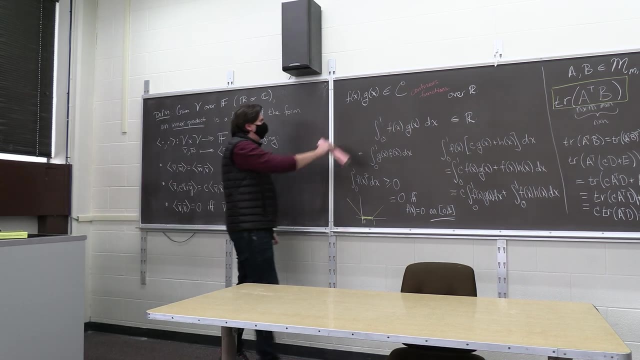 but? and all of our motivating examples were over the reals. so it makes sense why we would land at this, at this definition. but we have to be a little bit careful if we're working over the complex numbers because, as stated, this will lead us to a contradiction. 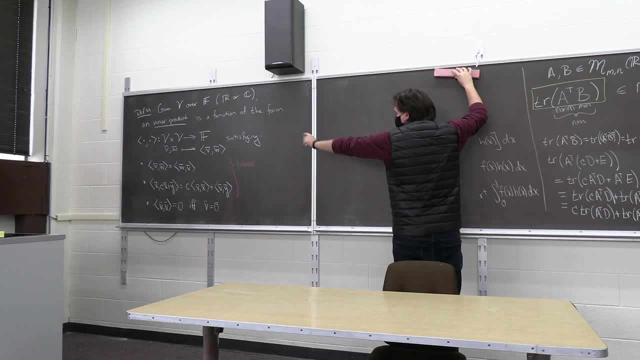 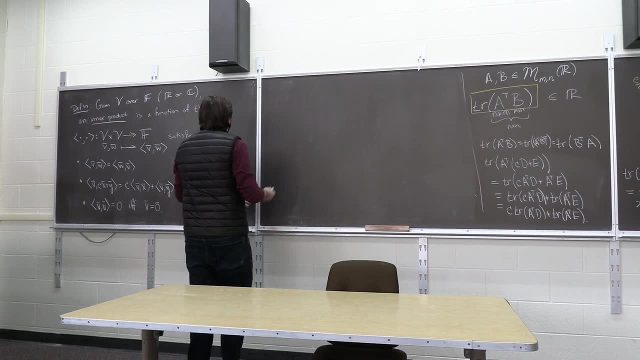 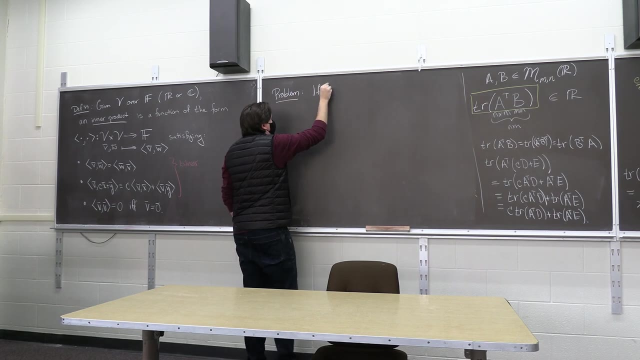 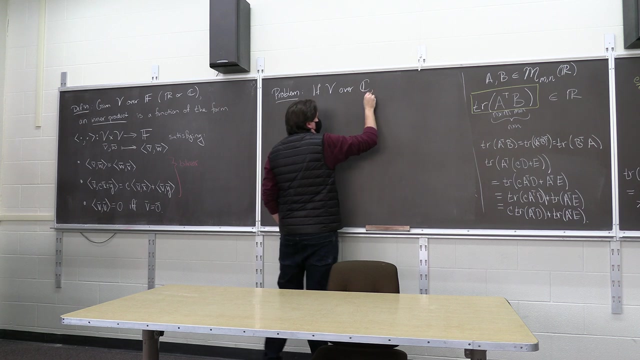 so let me show you the problem, and then we're going to slightly amend this definition, ever so small, to account for the fact the ground field might be v. so small problem. if v is some vector field over the complex numbers, then what you could do is you could take: 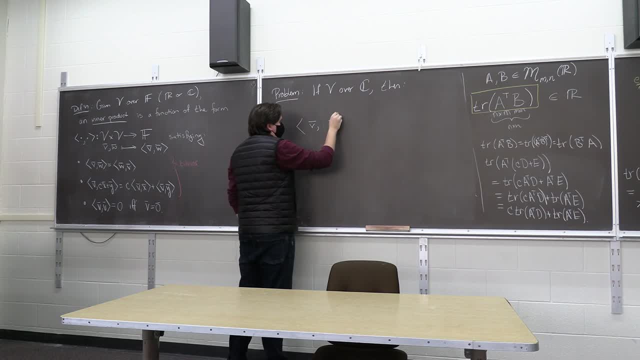 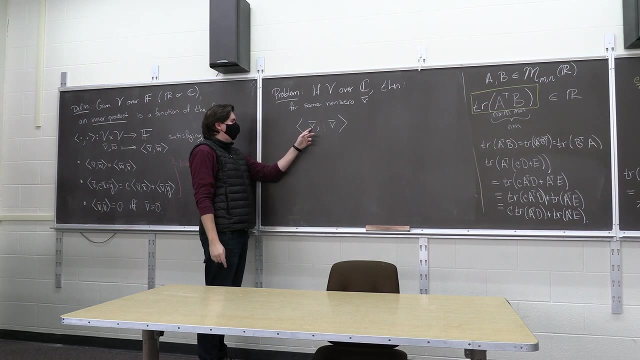 the inner product of v with itself. but what I'm actually going to do here, then, for some non-zero v, pick some non-zero v, instead of just doing the inner product of v with itself, I'm going to scale and multiply them both by the imaginary unit. 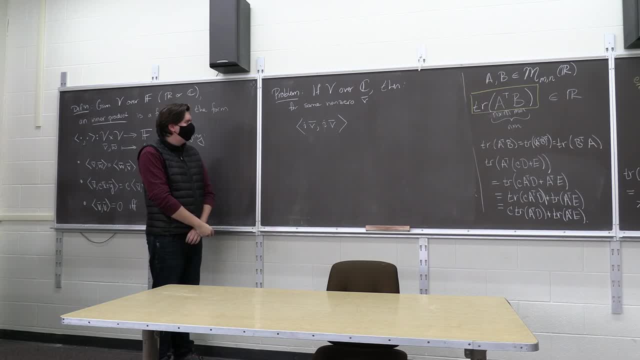 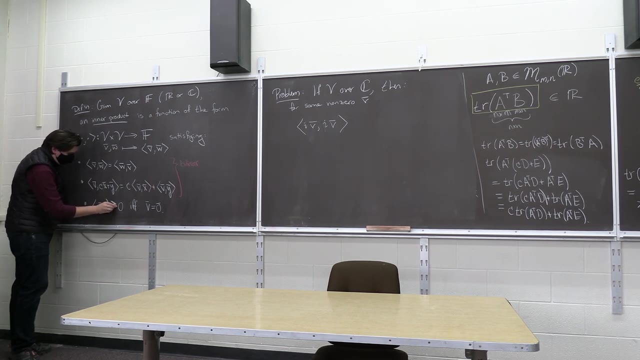 i well, if v is non-zero, i times v is still non-zero, so you have something with itself. so from the positive definite we have that: oh, this shouldn't say zero. this is greater than or equal to zero. right and only zero if v is zero. but since v is non-zero, 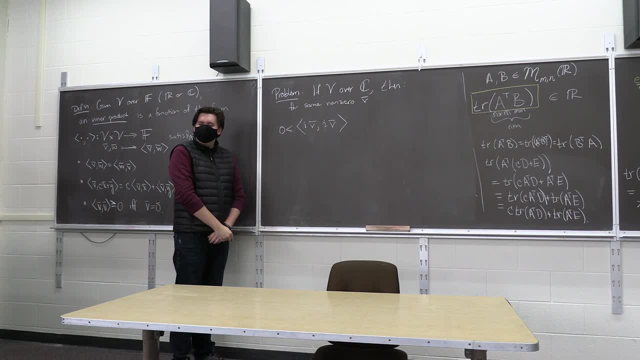 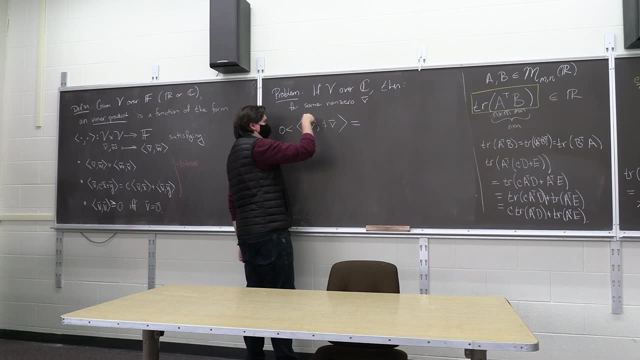 this should be positive, but then, since it's bilinear, linear in both the second and the first, we can pull the i out twice. so if you pull both those i's out, what do you have in front now? a negative one, right? so you get a negative one. 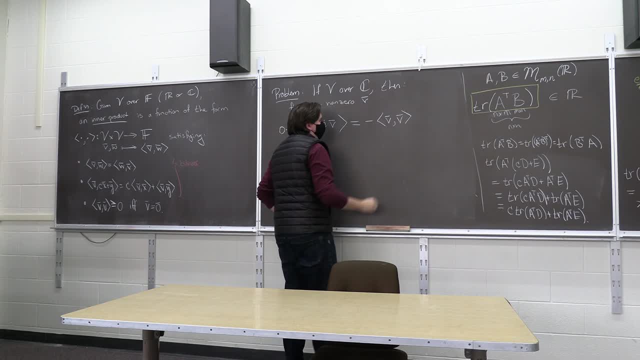 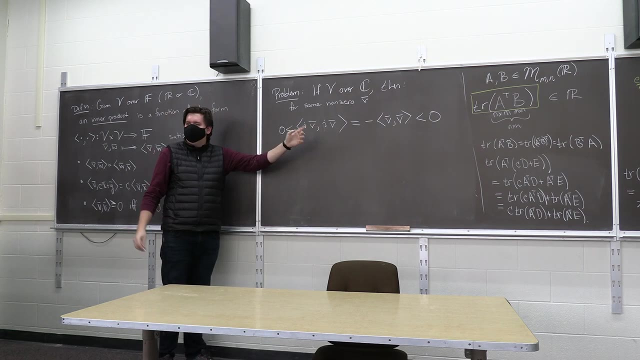 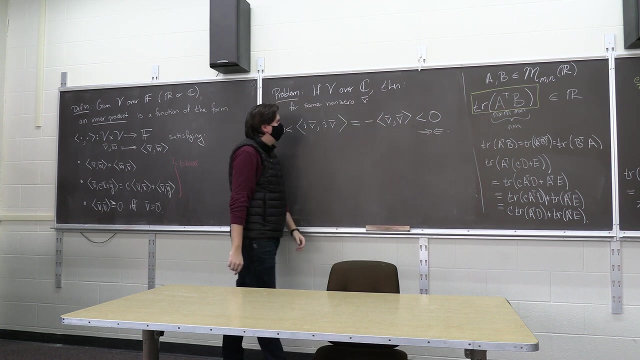 times v, v. we said v is non-zero, so the inner product of v with itself is positive, which means negative. the inner product of v with itself will be negative. ergo, zero is less than zero. like this is bad right, like not good. so what went wrong? 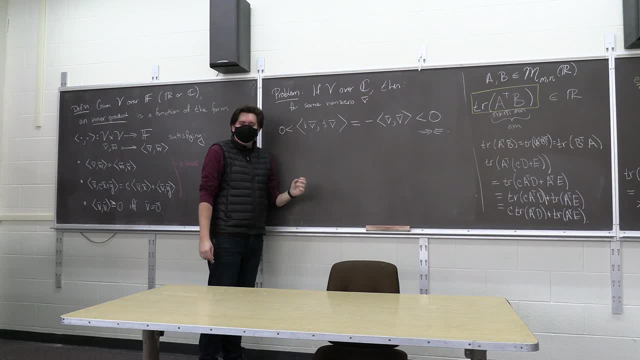 it's like: well, we're working with complex numbers, so there's some funny business there, and you might be like, ok, so something with complex numbers, what properties did we use? we used the commutative property, we used bilinearity, so there seems to be something. 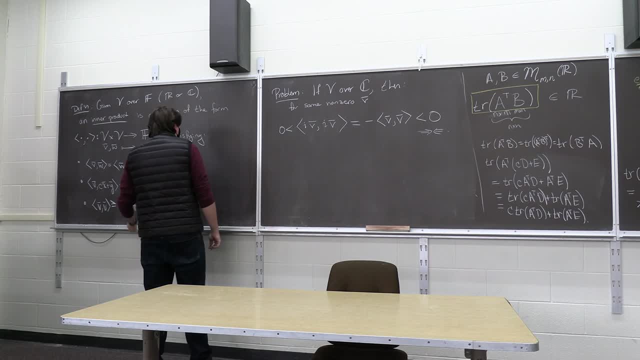 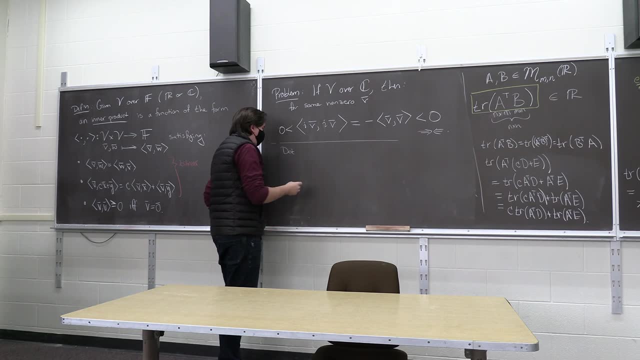 well, we used all three properties really, so we're going to have to append one of these like: how should we modify this definition? well then, we think back: how did you define, if you remember? how did you define the dot product over cn? do you remember if i have two vectors? 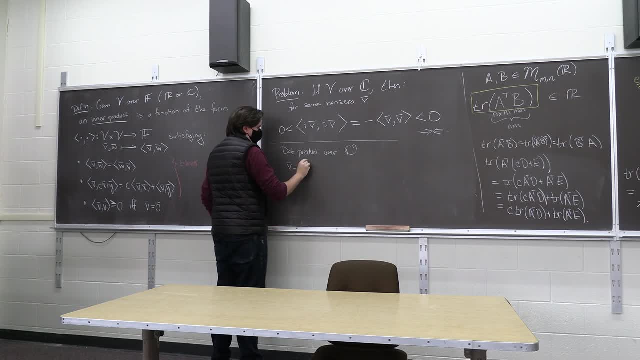 if i have some vector v, which is some, you know, v1 through vn, and some vector w, which is w1 through wn, how did you define v, dot, w? the same problem comes up in your first course on your algebra, and so you actually define this in a funny way. 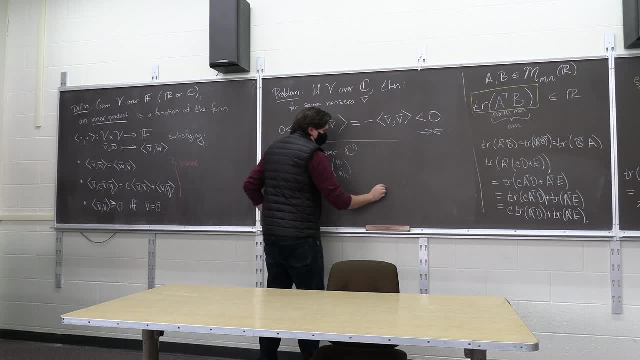 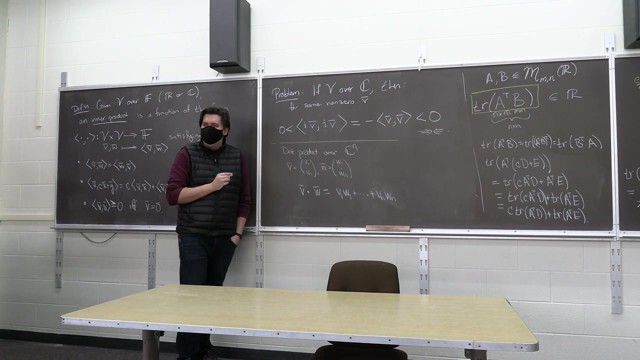 you don't define this. you don't define this to simply be the sum of the values vi. you don't write this. you don't write this as just v1, w1, up through v and wn and, like you know, you don't write it like that. 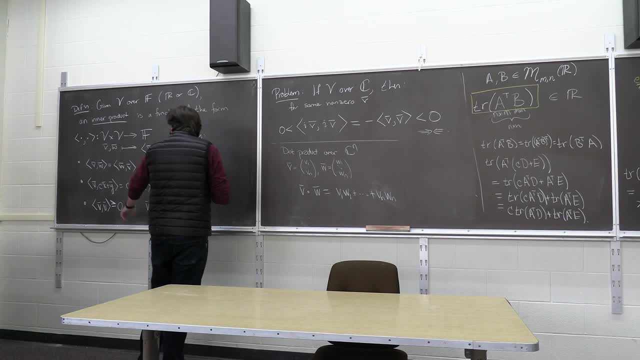 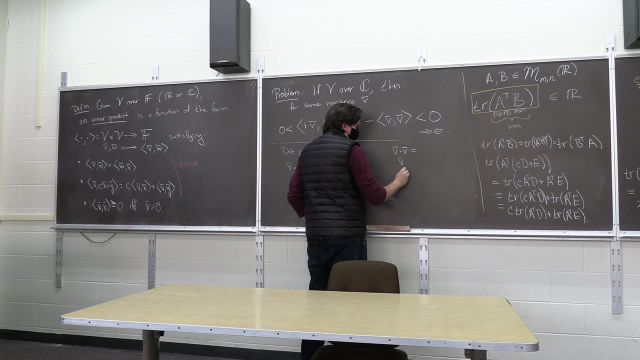 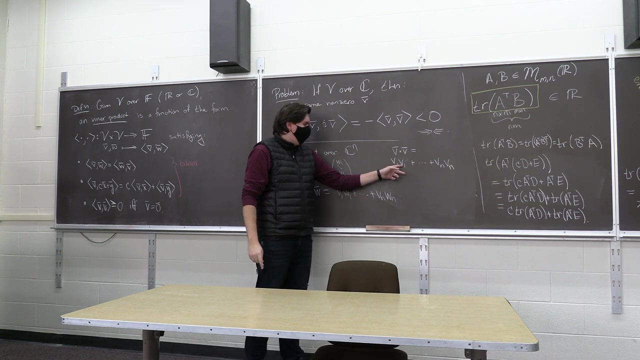 because you want this to be positive. definite like: what is v dot v? if it was just v1 squared up through v1 squared up through vn squared, that's not necessarily a positive thing. what if these values are i's? we're doing complex numbers now right. 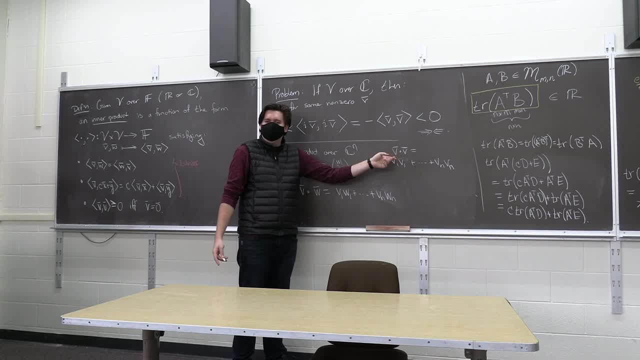 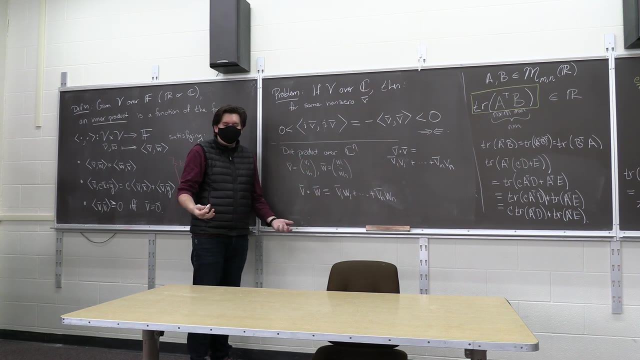 this could give you a negative thing. so how do you make sure that's a positive thing, right? you instead say: instead of multiplying them, you take the complex conjugate of one of them. now we're going to be super confusing, because this bar, i mean complex conjugate, this bar i mean vectors. 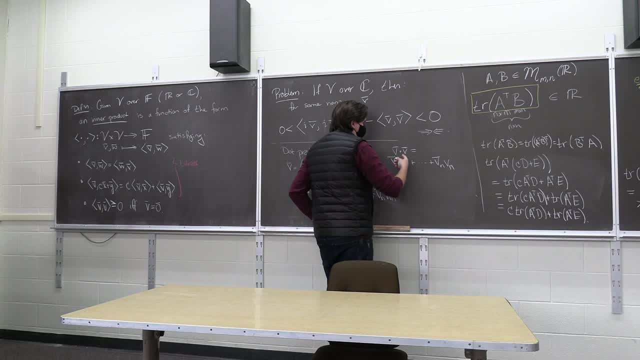 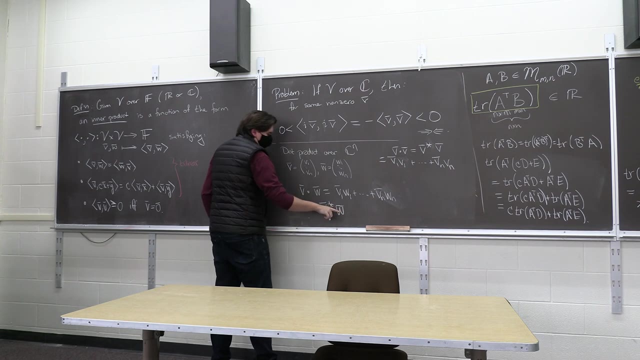 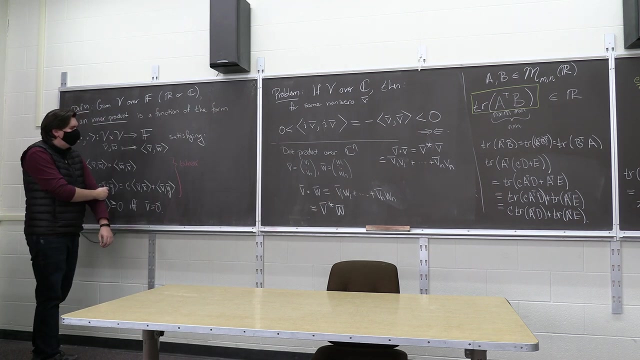 right, but what i'm saying here is: instead of: you don't define this as like v transpose times v. instead you do the conjugate transpose times v. this is defined to be v conjugate transpose times w. you take the conjugates of one of them, but now you don't actually have that it's. 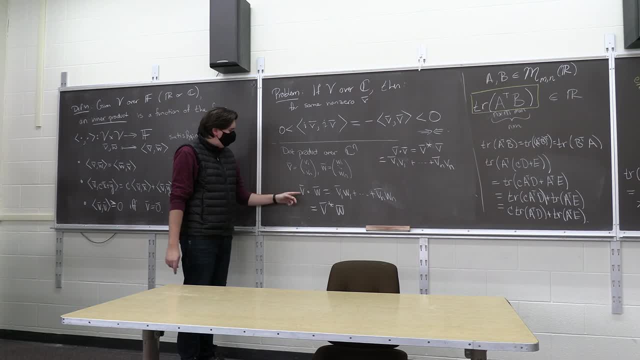 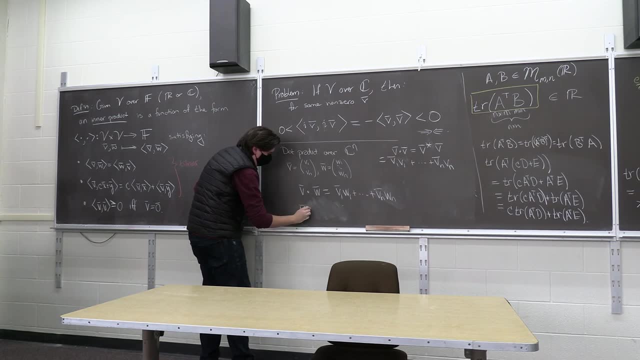 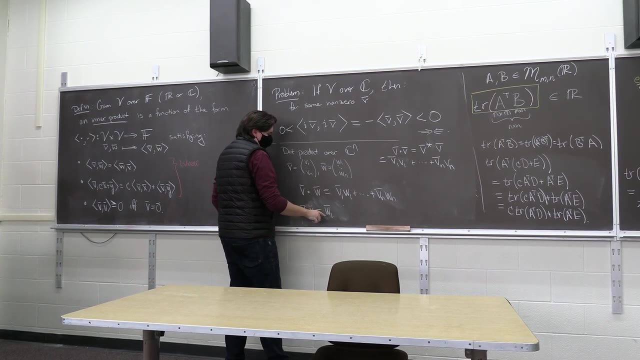 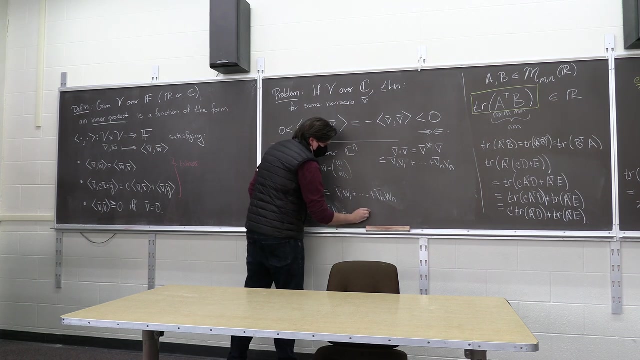 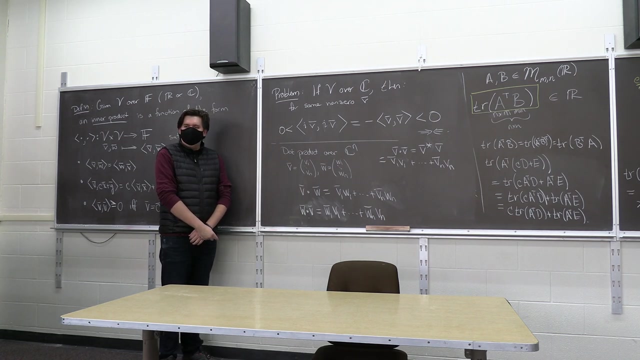 that it's commutative anymore because v times w comes out to be something different than w times v. w times v as vectors would be the conjugate of v1 times of w1 times v1, up through conjugate of wn times vn. these are not the same thing. 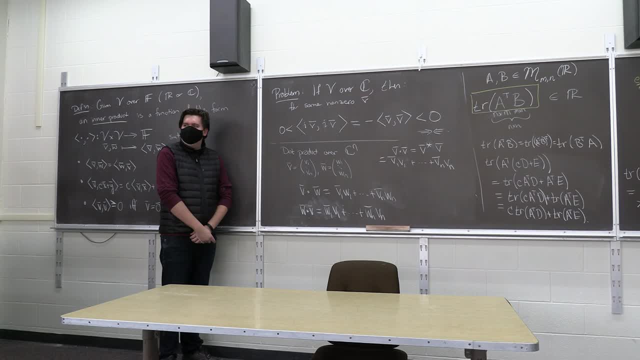 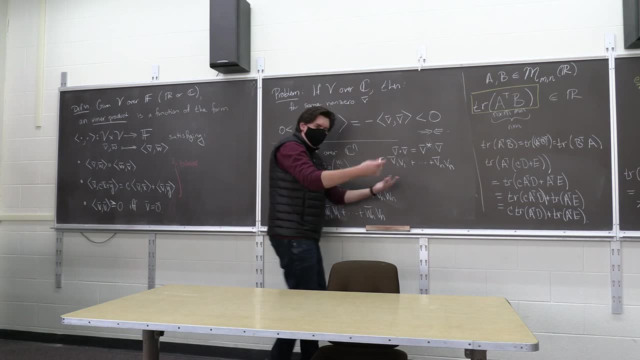 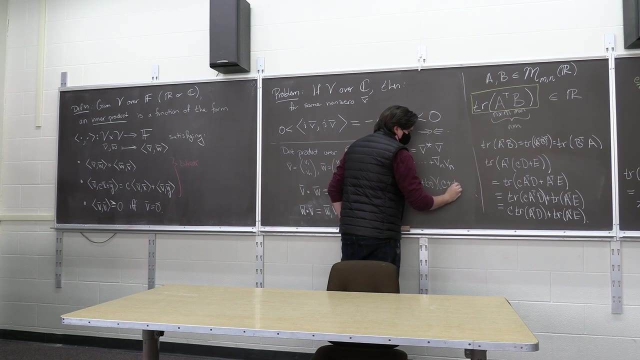 all right, we see these are different, but you know we, we know how complex multiplication works: a plus bi times c plus di. if you take the conjugate of the first one, you have a minus bi times c plus di. if you take the conjugate of the second one. 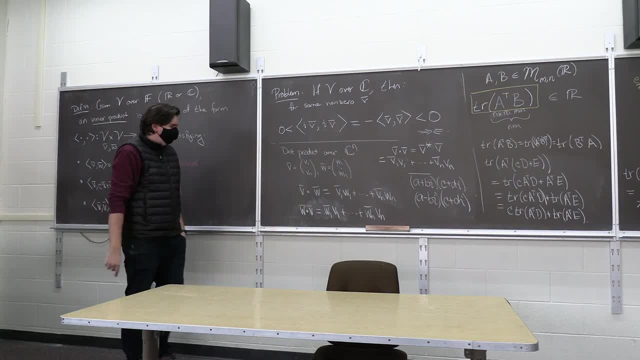 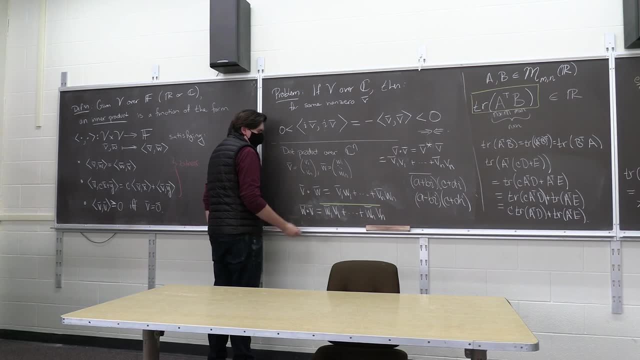 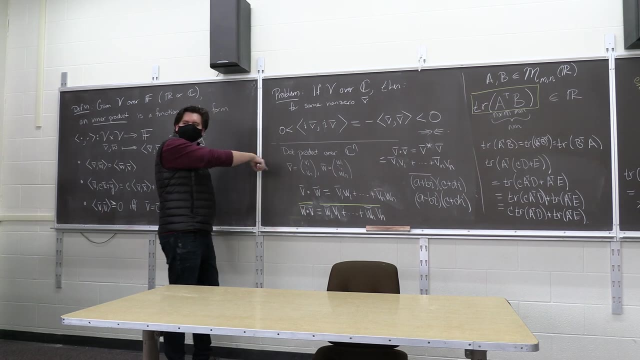 the minus would be there. right, it's different. so it's like: what's the relationship between these? well, this guy down here is the complex conjugate of the guy above him. so v dot w is the complex conjugate of w dot v, the complex conjugate. 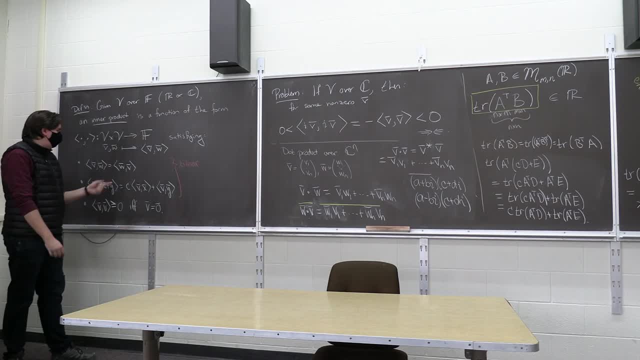 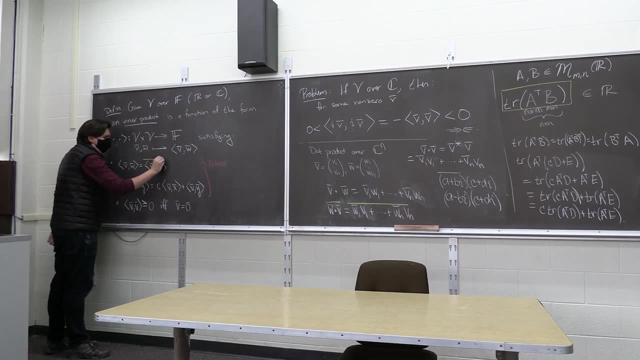 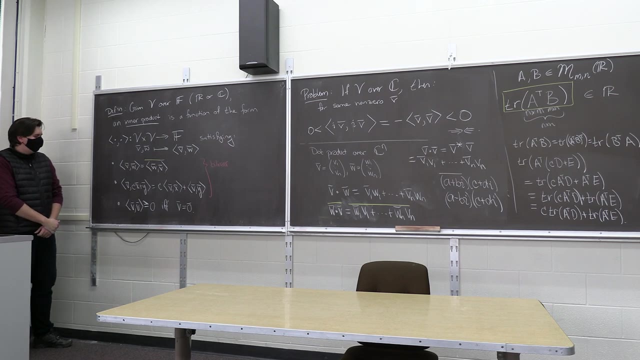 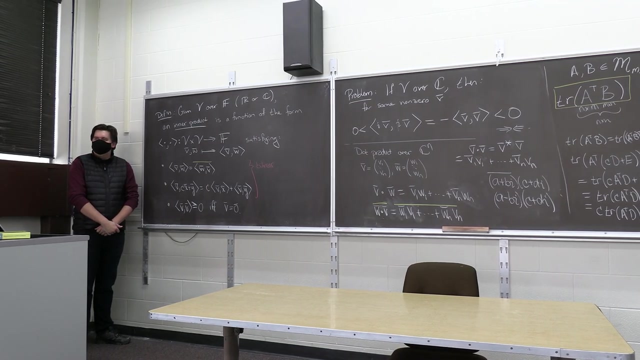 of each other, and so this is what we want to say here as well, that these almost commute. but if you're working over c, one is the complex conjugate of the other, and then this will all work out. oh, but wait a second if this doesn't truly commute. 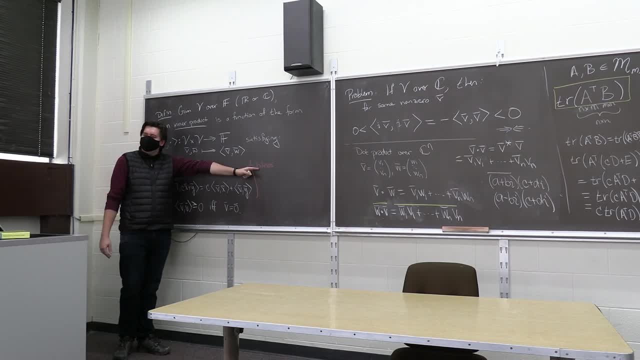 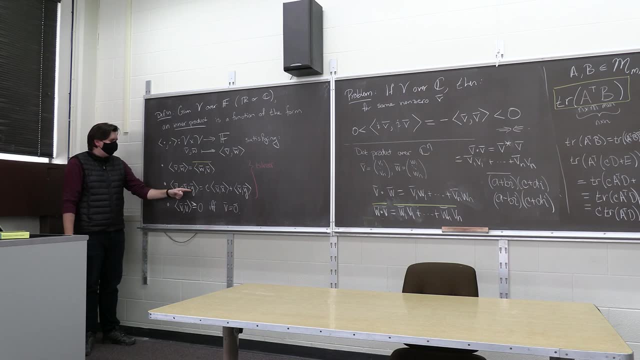 then maybe we can't recover that. it's bilinear, because in order to get those bilinear, we're using the fact that if it's linear over the second term, you can just commute it and it becomes linear over the first term. but now you have this: 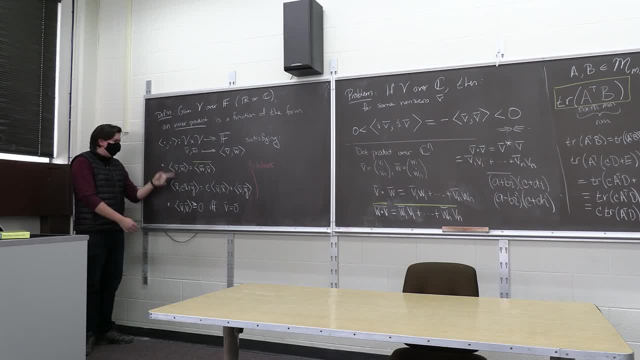 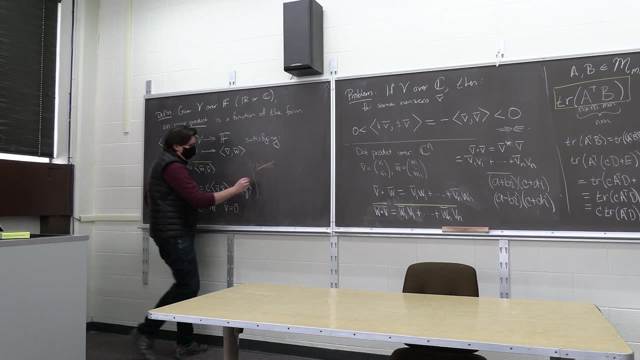 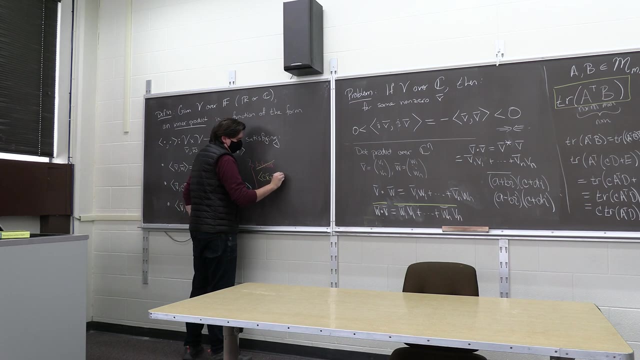 weird conjugate that comes in. so let's think about how these two properties combine. maybe it won't give us bilinear anymore. let's think about how these work together. let's say I want to have some cx plus y in a product with w. what will that equal? 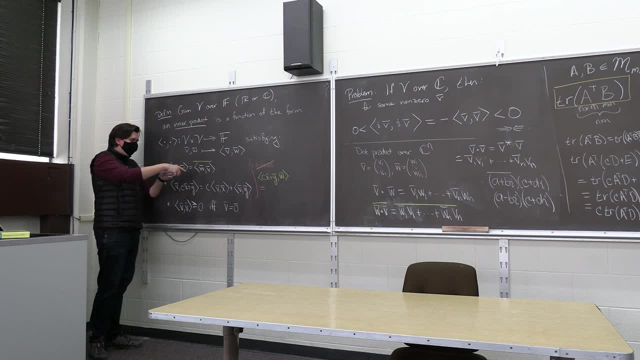 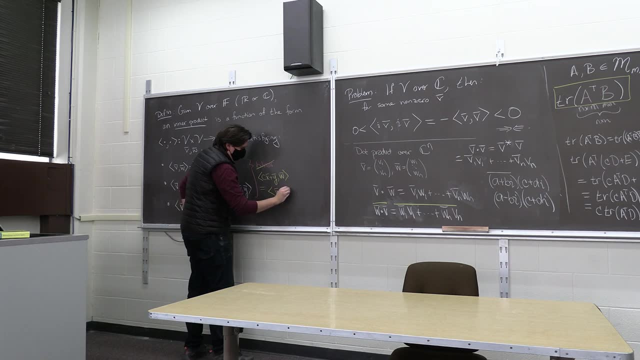 well, first I do my, I can commute, picking up, turn it into its complex conjugate and it becomes w, cx plus y, but it's the complex conjugate of it. and then I can use linearity on the second to say that's just c in a product. 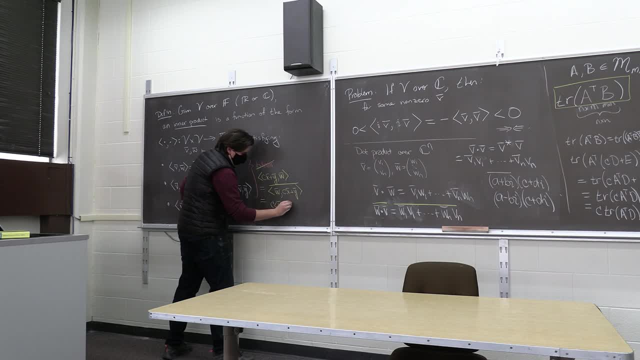 of w- x plus in a product of w- y, but it's still the complex conjugate of that whole thing. and then I'm going to commute this again, and so let's think about what happens. this is now going to change to x- w. it's going to become the complex conjugate again. 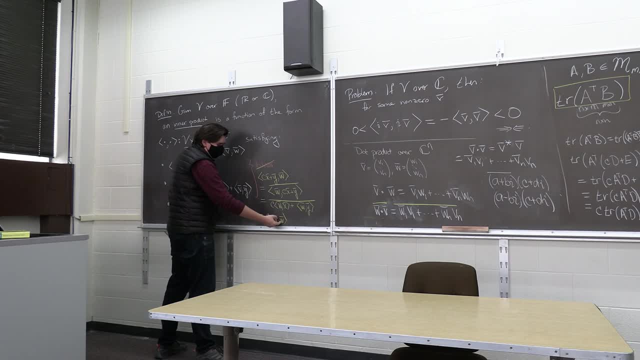 so you're going to have the complex conjugate of the complex conjugate, so he returns to his original form. the second guy, when you switch them around, will turn into its complex conjugate of the complex conjugate, so it's back to its original form. still is the complex conjugate. 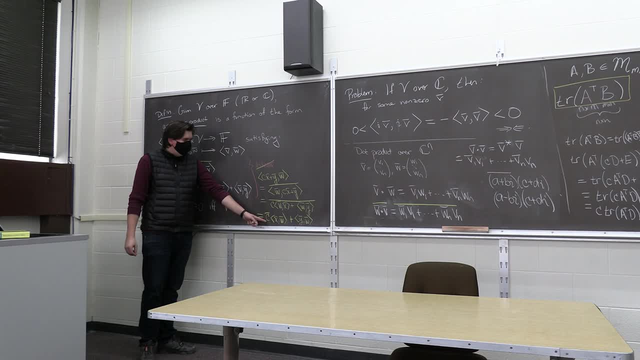 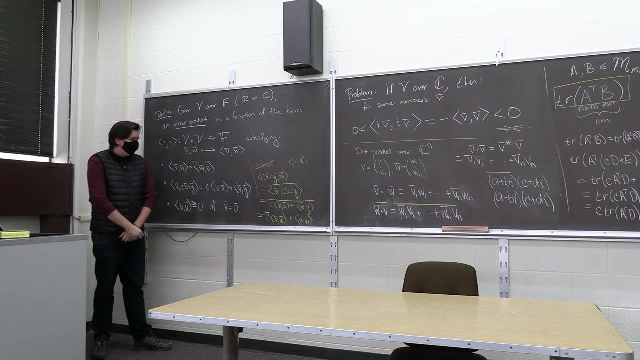 because c here could be some scalar in c. this is for some c in c. this is when we're working over c, so it's almost bilinear, except when you're working in the first argument. instead of just pulling the c out in the first argument, you pull out the complex conjugate. 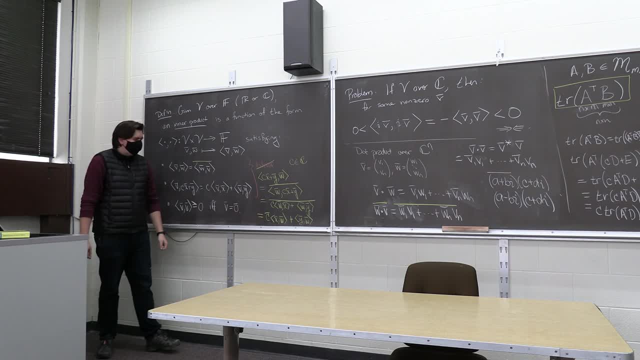 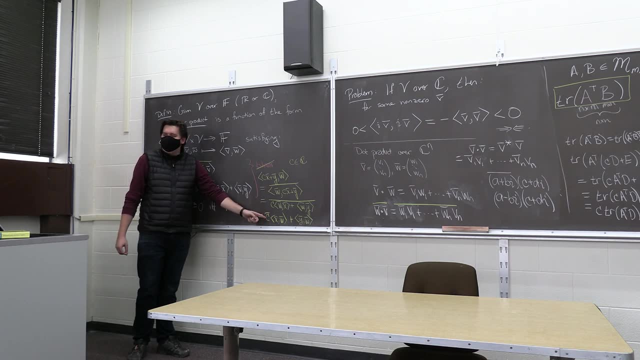 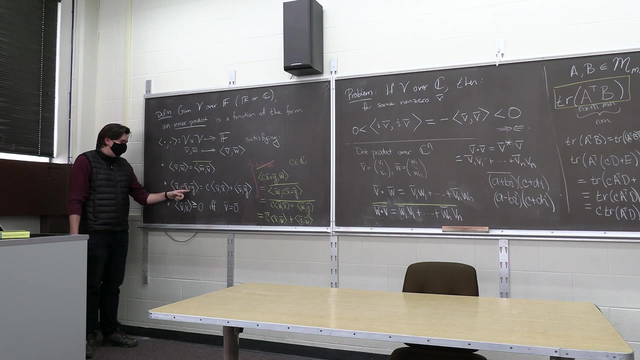 of c, so like it's really close to being bilinear, but it's not. it's linear in the second argument. but in the first argument c turns into the complex conjugate of c. so what should we call something? it's more than just linear in the second term. 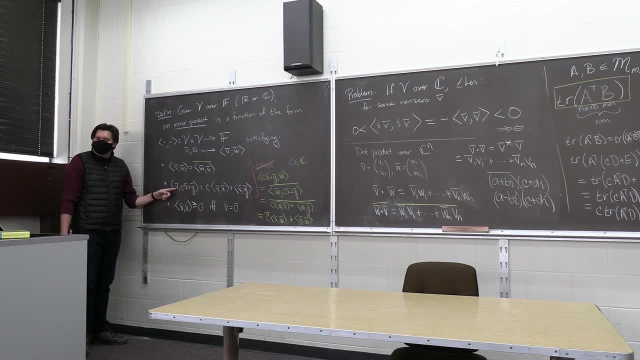 it's like linear in the second term and almost linear in the first term. it's like one and a half linear. so does anyone know the latin prefix meaning one and a half is Devin here. he knows latin. I think he went to some pretentious high school. 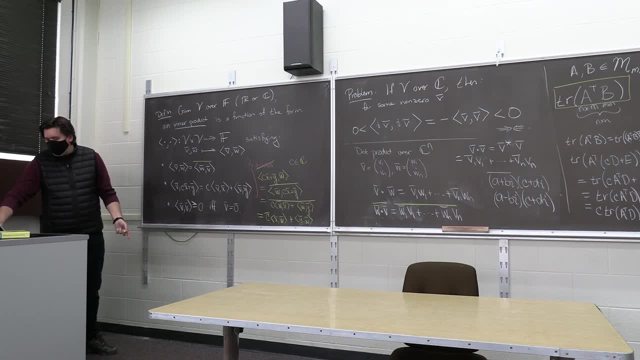 do? you guys know latin. so the university is about to celebrate our sesquicentennial. we were founded in 1874, which means that in 2024 we're a century and a half old. what's the word for century and a half sesquicentennial? 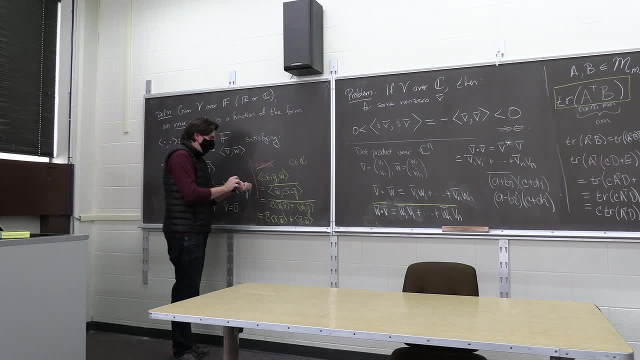 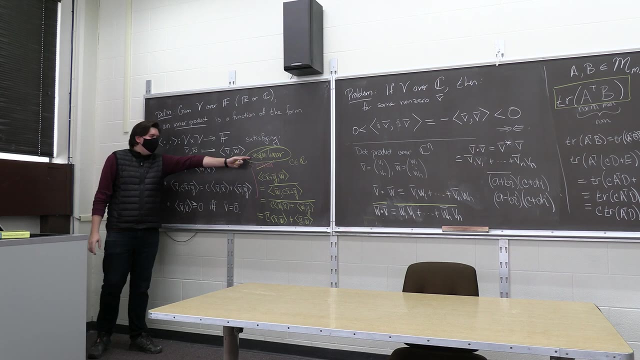 sesqui is latin meaning one and a half, so instead of calling this bilinear, we're going to call it sesquilinear, sesquilinear, sesquilinear. let me just emphasize: only have to worry about this if, working over the complex numbers, if your ground field is r. 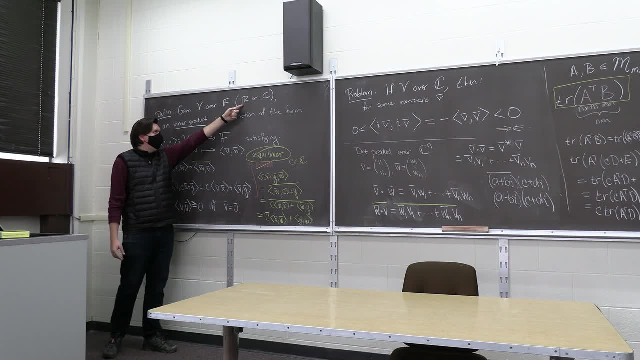 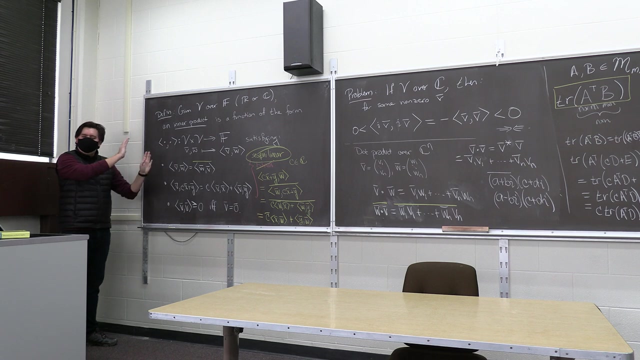 then the complex, the conjugate. there's nothing to worry about. it's the same thing. the c complex conjugate: over r it's bilinear, but when working over the complex numbers it's sesquilinear. so that's the definition, an inner product. We took a long time building up to this definition. 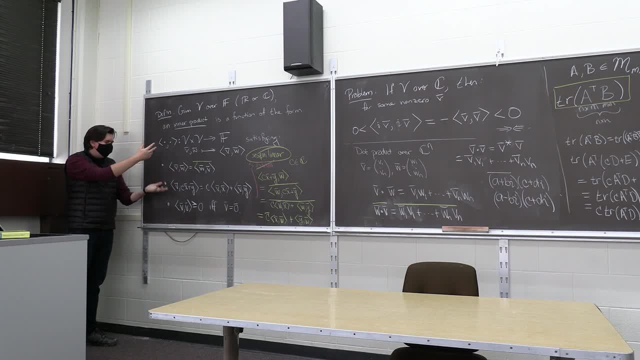 but I wanted to see lots of examples to try and motivate it and try to make it very clear like what this kind of thing is. It's like the dot product, but we can work with lots of other kinds of vector spaces too, If these are matrices. 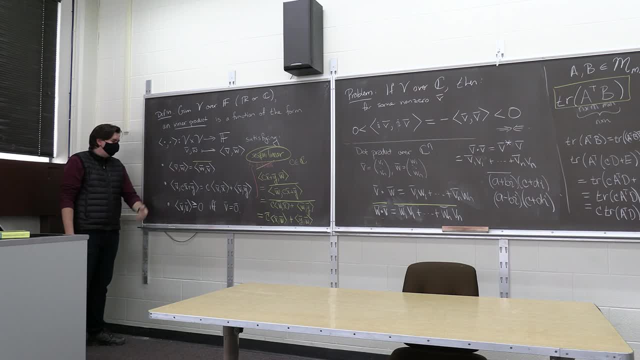 it could take the trace of the transpose of one matrix times the other. If these are functions, continuous functions- you can take the definite integral from some A to B of the functions times together. We'll look at some more examples next time, but let's stop there for now. 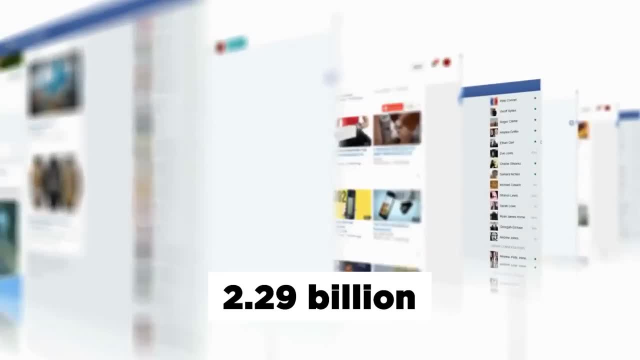 Did you know that Facebook removed 2.29 billion content pieces from their website after a record number of complaints regarding hacked accounts? Even the mighty Facebook cannot secure its systems 100%. Such is the situation when it comes to cybersecurity, Based on recent events and future. 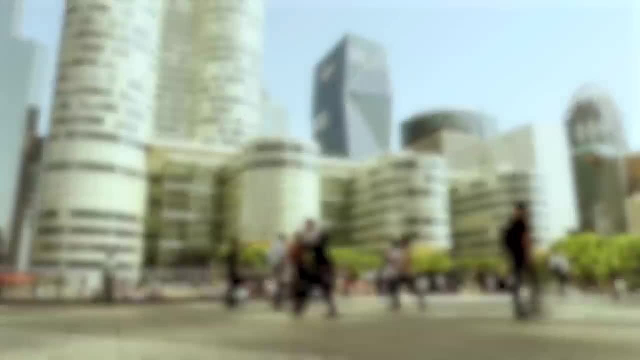 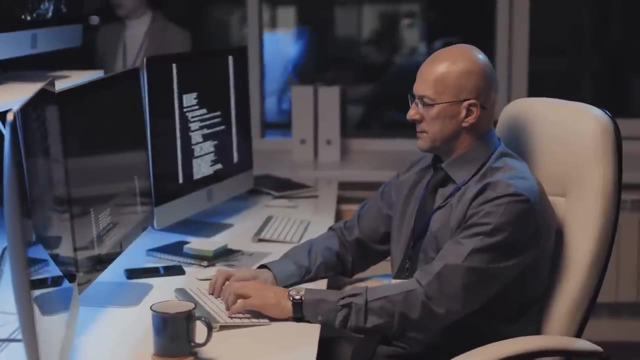 predictions, cybercrimes will cost organizations worldwide a whopping $10.5 trillion, coming from just $3.5 trillion in 2050.. So you can understand why it should not come as a surprise that professionals trained in cybersecurity are in sky-high demand and will be for the foreseeable. 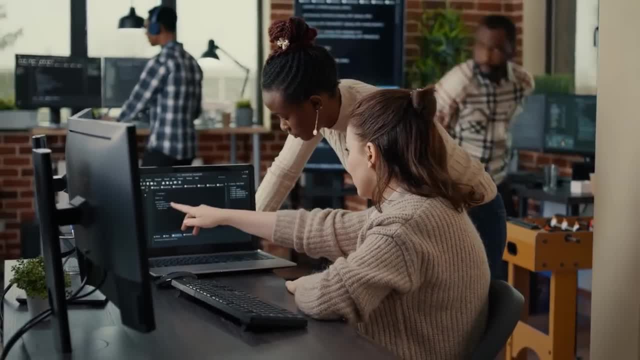 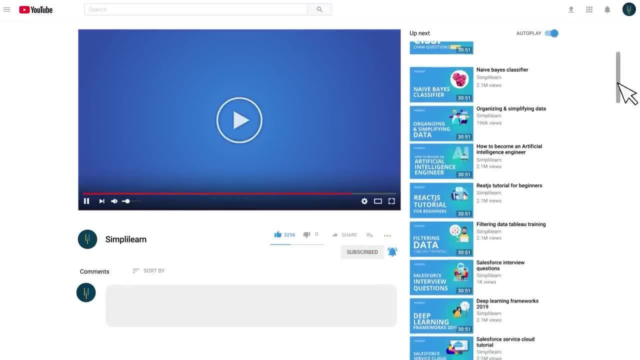 future. So what's better than staying ahead of the curve and getting trained in cybersecurity? Subscribe to it and simply learn. of course, since we upload tech-related content every day, Hit the bell icon to get notified whenever we drop a new video.